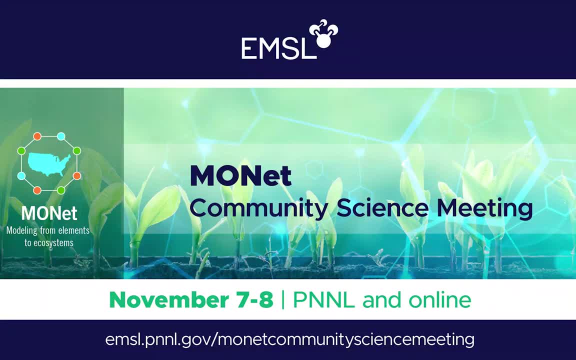 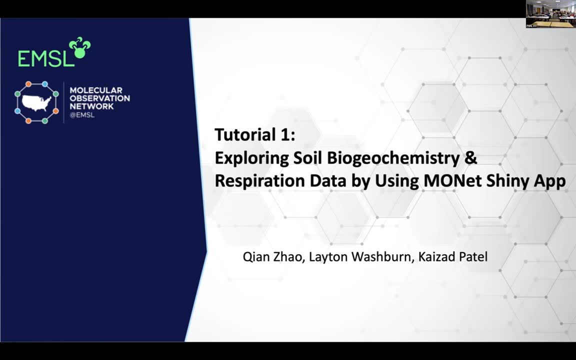 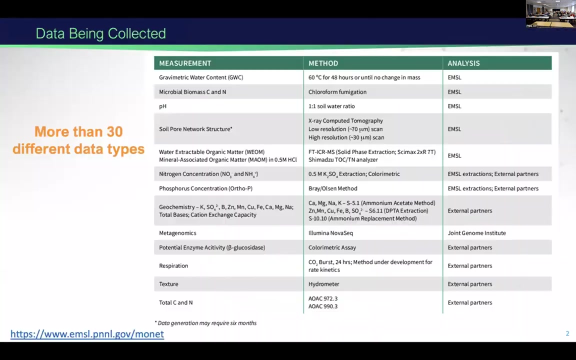 Here we try to show you how to explore this soil, biogeochemistry data, as well as respiration data, by using a training app that we developed here. as well as our approach can do further data interpretation, And I pull this data analysis table again to remind you of those different analysis. 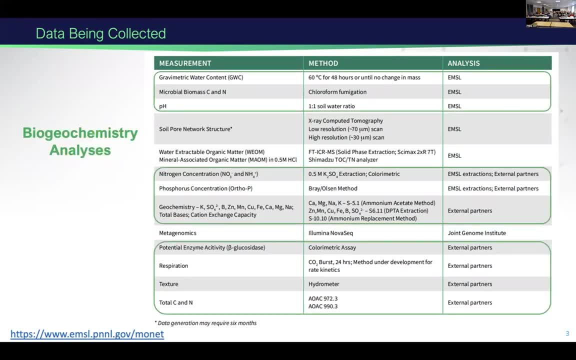 But for this tutorial we only focus on the biogeochemistry analysis, And next I'm going to give you a little bit details for each protocol that we use for each analysis. Maybe some of them is meaningless to you, but we want to emphasize those are the specific. 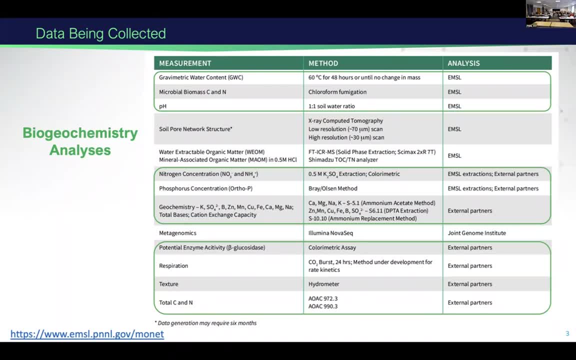 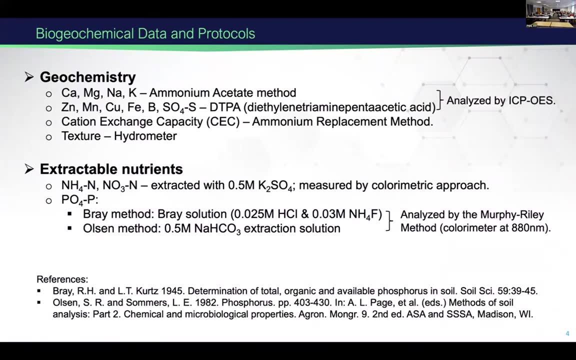 protocol that we use to generate those data And I group this analysis into four categories. First is a geochemistry data. So for the first four ketones, we use this calcium, magnesium, sodium phosphate. We use the potassium, We use the ammonium acetate extraction to get the extractant solution and measure by. 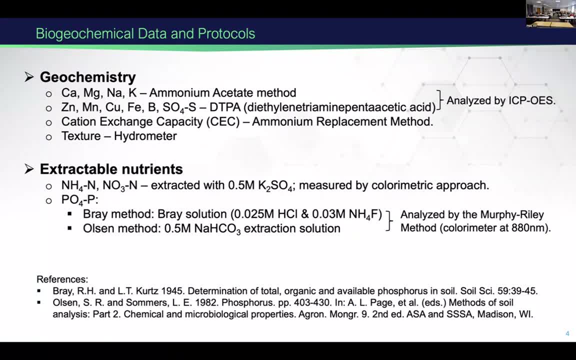 ICP-OES And the other group of the ketones. We measure by this DTPA acid and measure by ICP-OES as well. Of course. we deliver this ketone exchange capacity that's measured by this ammonium replacement method. 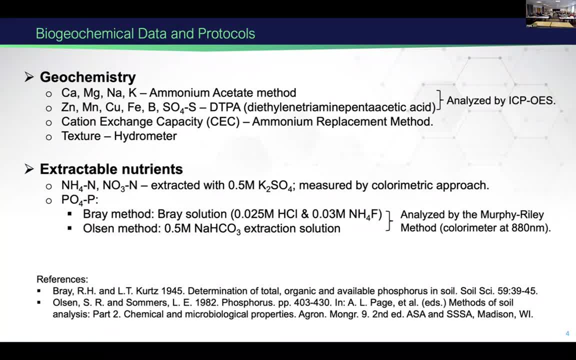 So we use ammonium acetate to extract those soil particles and the ammonium going to replace those exchangeable ketones from the particle surfaces And then we use the HCL to further replace this ammonium off the surface and measure with the color metric approach to measure. 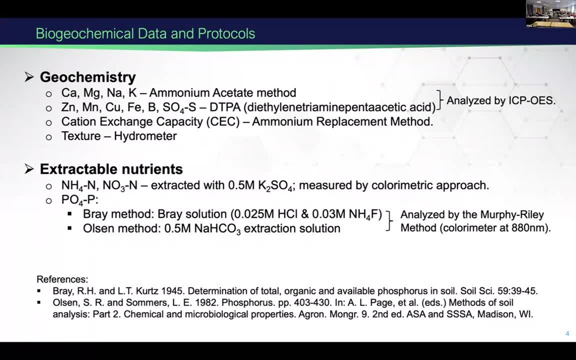 And then we use the HCL to further replace this ammonium off the surface and measure. to measure the ammonia concentration, which can be calculated to the ketone, the CEC value, And for the texture, we measure the percentage of the sensitive clay by hydrometer. 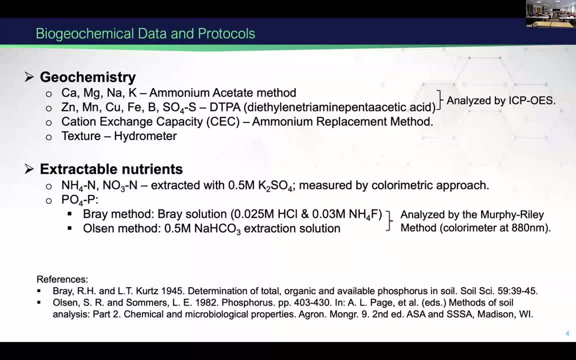 The second group is the extractable nutrients. We use K2SO4, potassium sulfate to extract this inorganic nitrogen and measure it by this color metric approach. For the phosphor, We use two different methods. The first method, depending on the pH of your soil. if that's below nutrient, we use a brine. 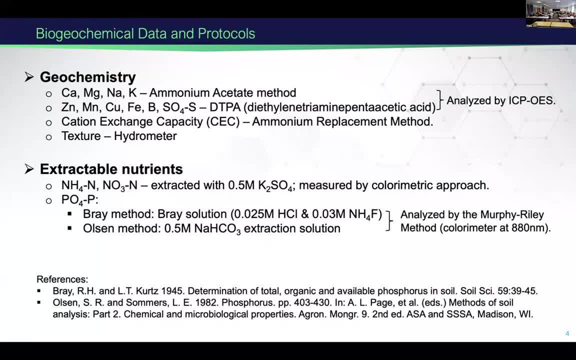 method. The solution is a mix of the HCL and the ammonium fluoride. For the pH above nutrient, we use this sodium bicarbonate to extract it, and both those extracted solutions are measured by this Murphy-Reilly method. So we have this classic, highly cited reference down here to support those. 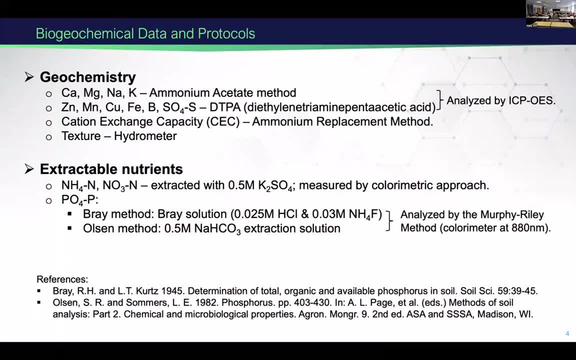 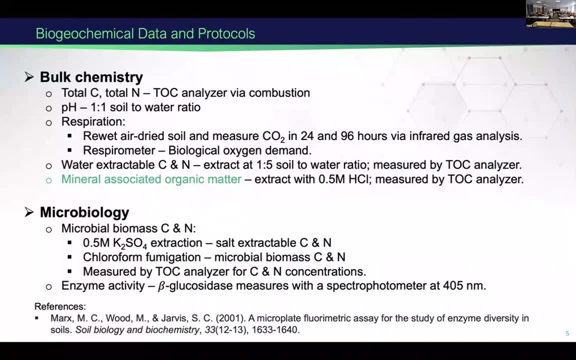 And the next group is the bulk chemistry. So for the total carbon-nitrogen concentration we use the TOC analyzer. For the pH you may use different ratios, but here we chose the one-to-one soil-to-water ratio And the respiration. for the 1,000-soil pellet study we use this rewet, the air-dried soil. 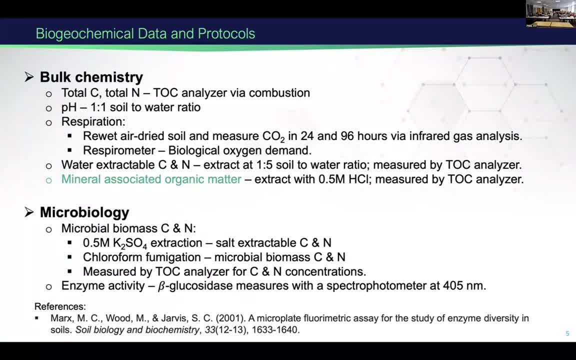 and measure the CO2 in the high space for two hours And then we use the HCL. We use the HCL, We use the high space for 24 hours and 96 hours by this infrared gas analysis, But from the feedbacks from users, modelers and also our scientific advisory committee. 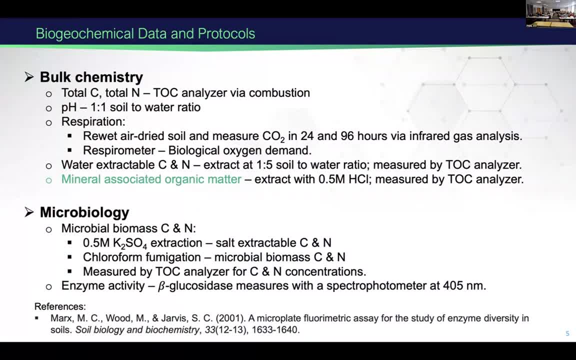 members, we hear that there is a strong need to have this kinetics data for the respiration that can be helpful for the data interpretation and the modeling works. So for this first year of the MONAT samples, we used this. We used this respirometer to measure the CO2, cumulative CO2, over five days. 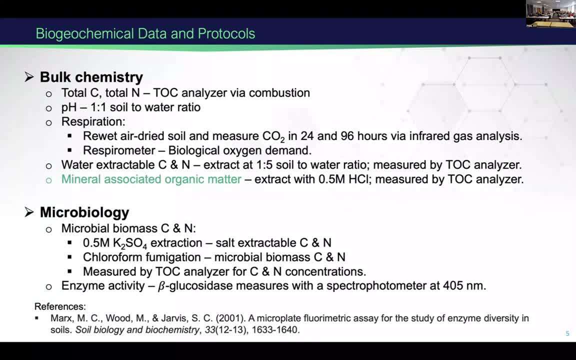 So that will give us the power to fit those respiration data with the curves based models and to do further interpretation. So for the next part of this talk I'm going to dive a little bit deeper to this respiration method, how we process those data and give you the final data products. 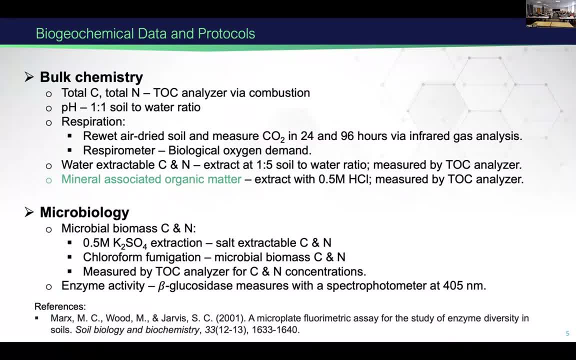 Dr. Okay, Thanks. So another bulk chemistry is the water extractable carbon-nitrogen concentration that we measure by one to five soil to water ratio and based on TOC analyzer, And same to this new analysis we had this first year is a mineral associated, organic. 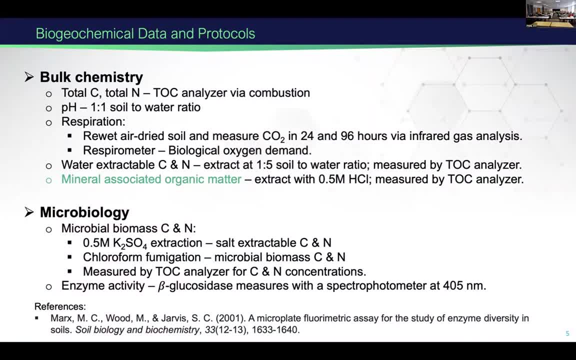 matter extracted by 0.5 molar HCL. So that represents a weakly bound organic matter to the mineral surfaces. But also, we are under development. There are more harsh solvents, Dr. Okay, Thanks, So we know that the HCL is a mineral cause. 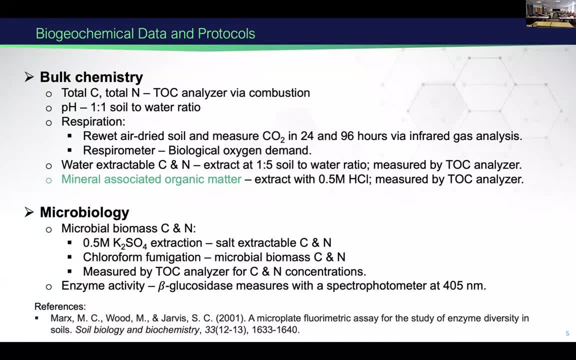 We know that the HCL is an organic matter, So we're going to use the HCL to measure the HCL, and the HCL is an organic matter. We have a lot of different samples, But what we're doing is we're going to be using the HCL to measure, the HCL to measure. 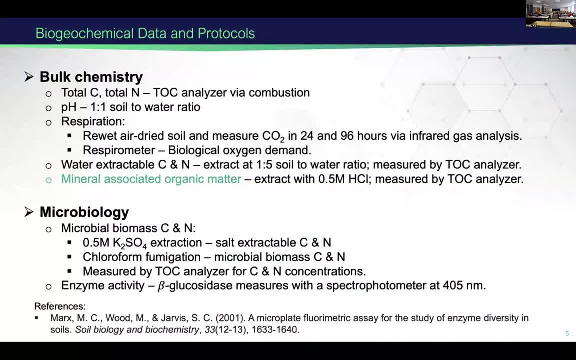 the HCL and the HCL to measure the HCL And we can see that we have these two samples here And we can see that the HCL can be extracted, can extract those soils to give you a different pools of the stable carbon. 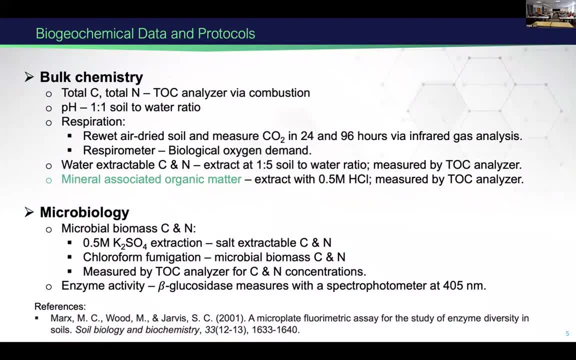 And, of course, both of those extractions have been measured on FT-ICR to give you the power of this molecular composition, Dr. Okay, Thanks, Dr. The last group is the microbiology. have this microbial biomass carbon nitrogen been measured by this sequential extraction? so we have. 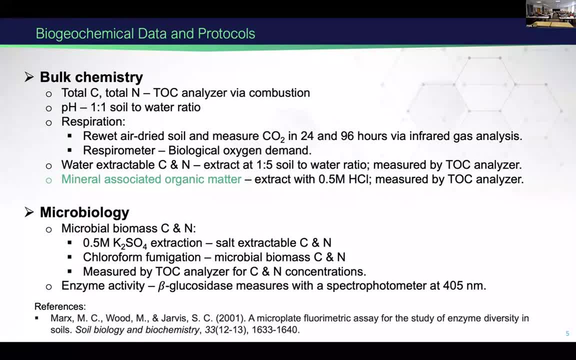 this k2so4 to extract this salt, extractable carbon nitrogen and chloroform fumigation to lyse the cells and to release those microbial carbon. so measure this microbial biomass carbon nitrogen with toc analyzer. so, lastly, as the this enzyme activity, we use this microplate follow metric. 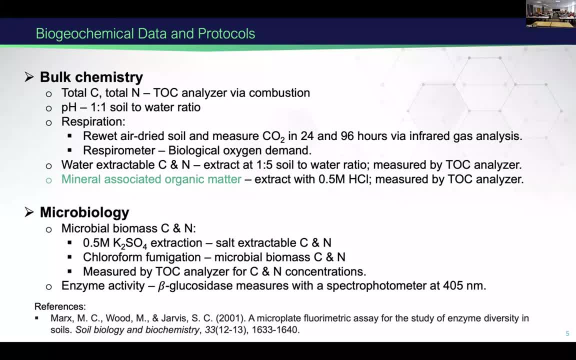 approach to measure this beta glucose, of this potential activity. so i want to emphasize that all of this protocol is under the discussion with experts in different domains and also our users. they got feedback from them to make this final decision. decision on each particle and uh, yeah, that's uh, with a strong justification from the literatures. 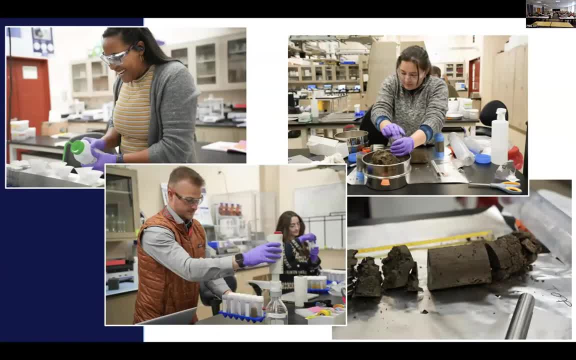 and of course, those uh, uh heavily labor intensive work couldn't be happen with all these happy faces in our labs. so we have a group of lab members to help us to process, uh conduct those analysis, process the soils through sieves, to make all those data products available and possible. 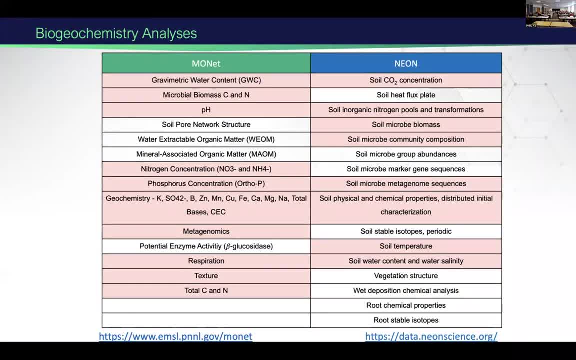 we'll come back to this list again. this is all the biogeochemistry data we provided, and i know that's a lot of data we are using, but we are doing it for the purpose of understanding it. come back to this list again. uh, this is all the biogenic chemistry data we provided, and i know that is a lot of data we are using, but we are doing it for the purpose of understanding it. 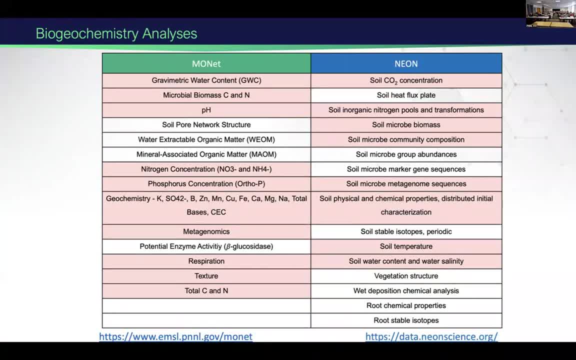 this is kind of a common data type that most of you can do in your own lab or other networks. Here I use NEON as an example to compare with our biogeochemistry data, So you can see the highlighted analysis overlapping between MONAT and NEON database. 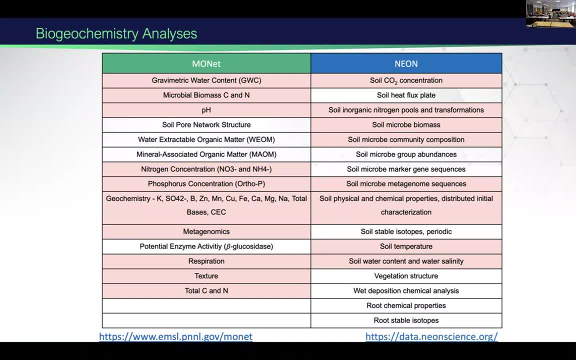 So again I want to emphasize, we want to have our own standardized protocol for each of these analysis So the data in this database can be compared across different sites, different ecoregions or even over multiple years down the road. So we have this. 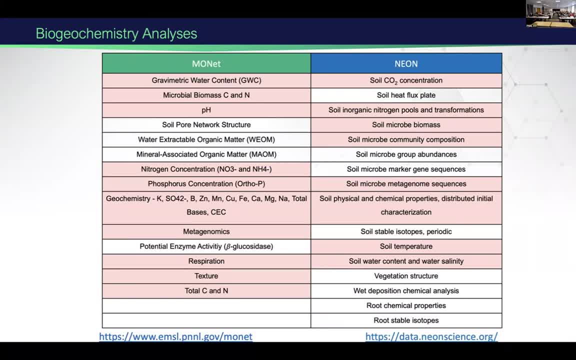 SAMANSA, representing NEON network. So we partnership with them to get some soil cores from the NEON network. But this is not the full list of their analysis. They have a long list, including the atmospheric data, plant phenotype data as well. 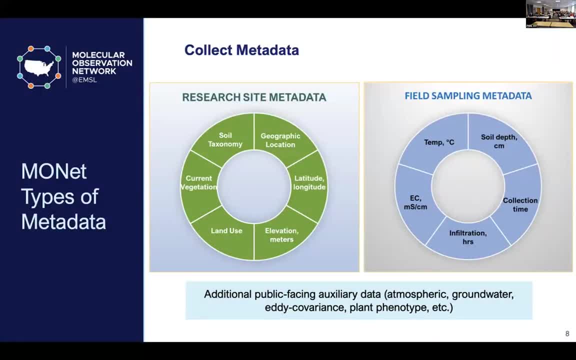 So, along with those analysis data, we also collected the metadata, including the research set metadata, field sampling metadata such as soil taxonomy, latitude, longitude, soil depth, land use test. Those data are also useful to be used to gather with our analysis data to do further interpretation. 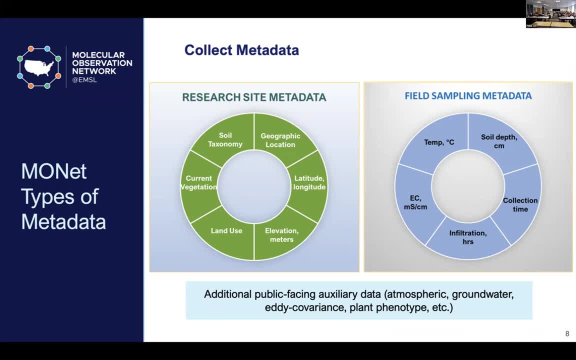 And some of those sites also have other data available, as I show down here, like atmospheric data, groundwater plant phenotype data. Those are collected by each individual PIs in their own research project, But they also ask for access to those public data sets. 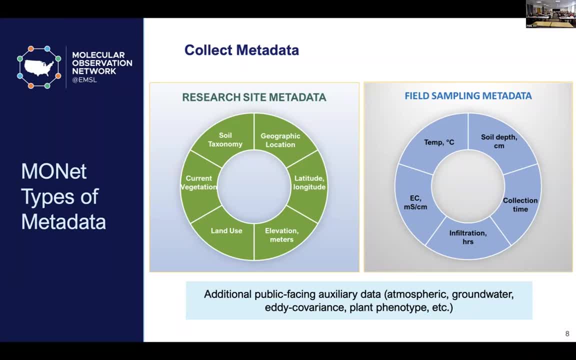 So if you are interested in those other data, you can reach out to me, to any of our MONAT members, so we can build connection with those PIs. And some of them are like an open public repository: You can directly access to those. 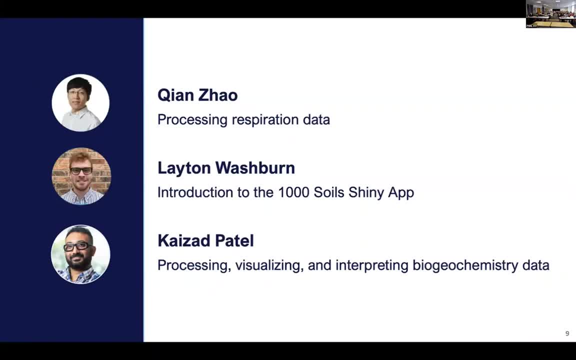 So with that, for the rest of this tutorial, we're going to break into three different sections. First I'm going to dive deeper into the respiration data to show you how we process it, And then Leighton is going to come after to give you an introduction. 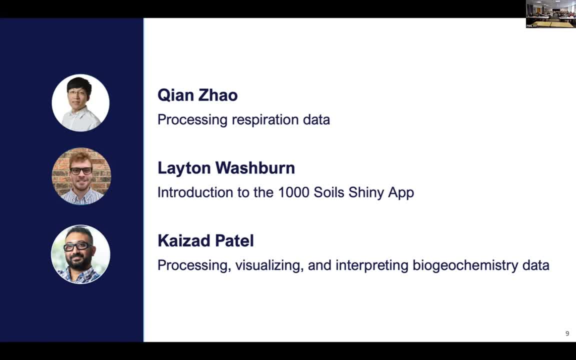 to the SHINee app to show you what those functions on the SHINee app can help you to explore those biogeochemistry data. And Kaiser is going to use the R-script to further explore the data but also interpret this data for scientific meanings. 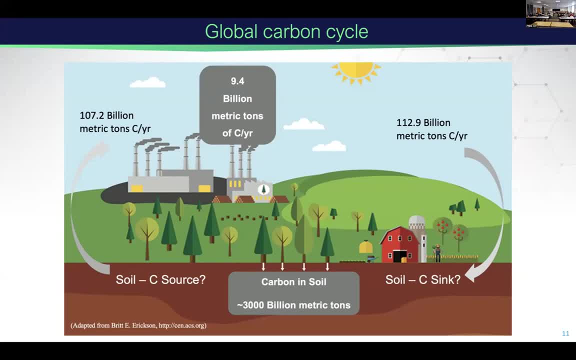 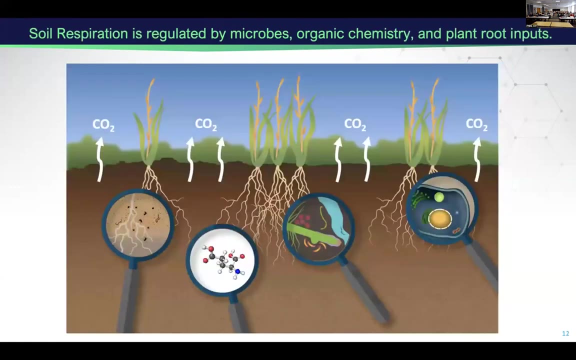 So here I give you a big picture of the global carbon cycling. and soil is one of the largest carbon reservoirs on Earth, So it's important to sequestrate carbon from atmosphere, but also release carbon to it as a respiration, And the soil respiration can be regulated by so many components. 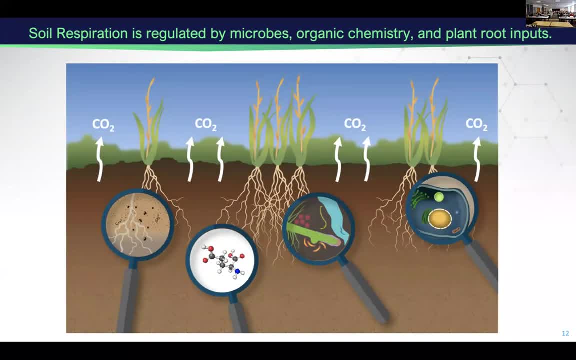 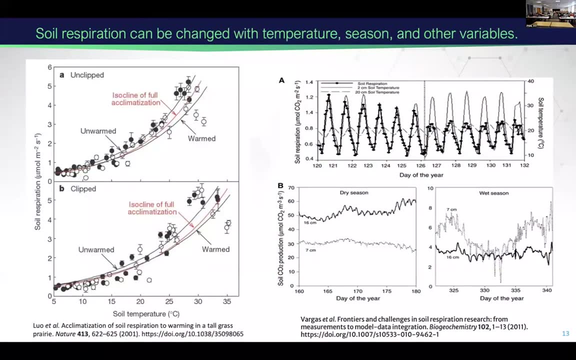 like microbial communities, organic matter, chemistry, as well as the plants' roots inputs. There are a lot of studies done on the soil respiration. Here I'm just showing you a couple of examples. The one on the left is how this increasing temperature can increase the soil respiration. 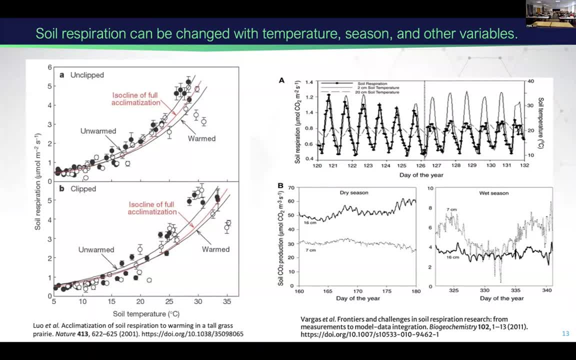 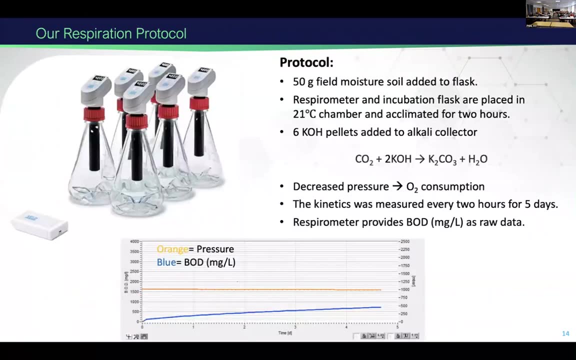 The one on the right, to show you how the respiration being changed over time, over seasons- And I'm going to give you a great case study this morning- as well as how this wildfire intensity effect on the soil respiration as well. So here is our new protocol to measure the respiration with this respirometer on the left. 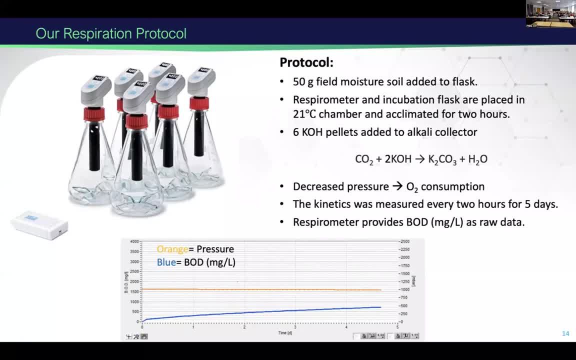 So we have this flask that incubated with 50 grams of the field moisture soil and with a respirometer installed on the top. It placed that into a 21 degree C chamber and let it liquid burn for two hours and start the incubation. 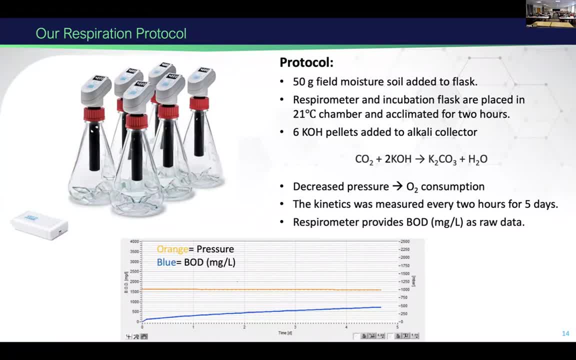 We measure every two hours up to five days In this respirometer. we have this collecting collector. we put six pallets Of the KOH in it, So that need to react with a CO2 from soils to produce this potassium carbonate and water. 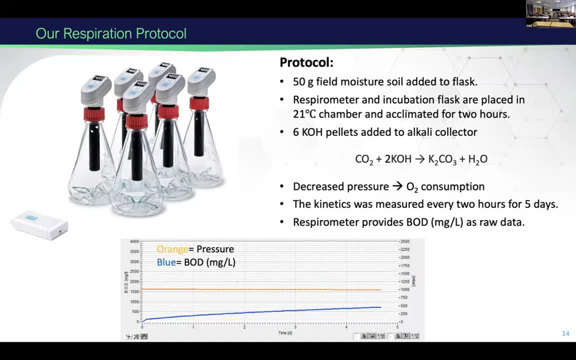 Basically it converts CO2 into water And those oxygen consumption from the high space will convert to water and cost measured by this decrease the pressure. So here is a screenshot of our software To give us a raw data that convert from pressure to the biological oxygen demand. 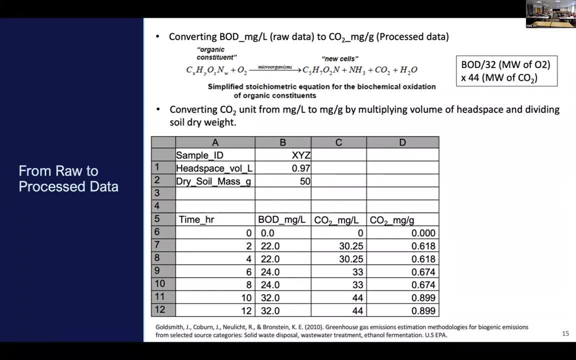 So then, once we got this raw data in BOD, we further converted to CO2 production By this simplified sticky geometry equation to represent the biochemical oxidation of organic compounds in soil. So here is a generic reaction, just representing one to one: oxygen Consumption to CO2 generation ratio, molar ratio. 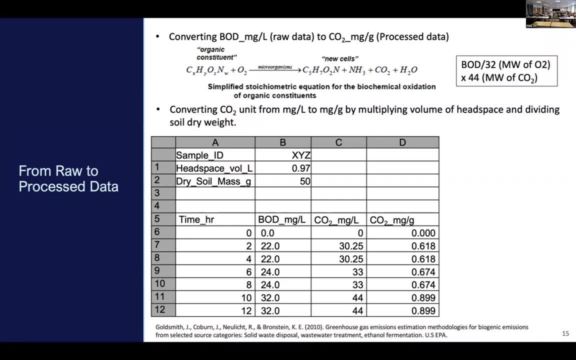 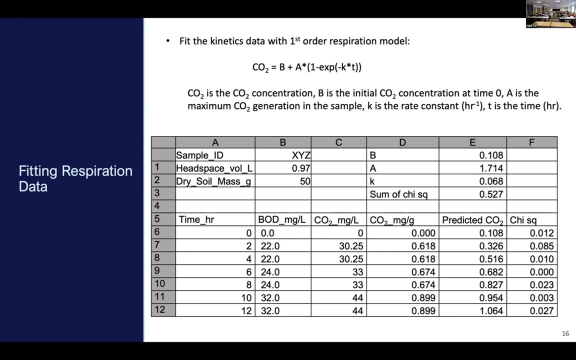 And we can do the conversion based on molecular weights of those two. And we further convert CO2 from a milligram per liter to milligram per gram By including the volume of the high space and the soil dry weight. So with those kinetic data we further fit to this first order respiration model. 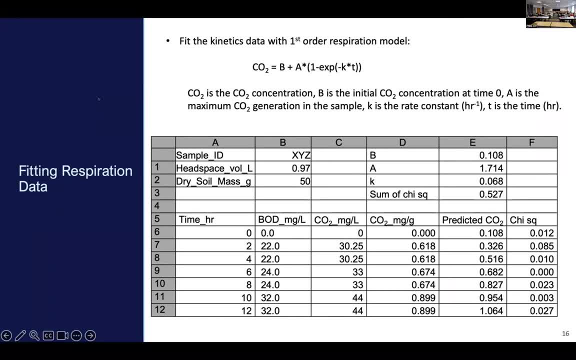 If you are not familiar with it. This CO2 represents Our measured data and B is the initial CO2 concentration at T0.. A is the maximum CO2 concentration when they reach to the plateau and K is the rate constant and T is the time in hour. 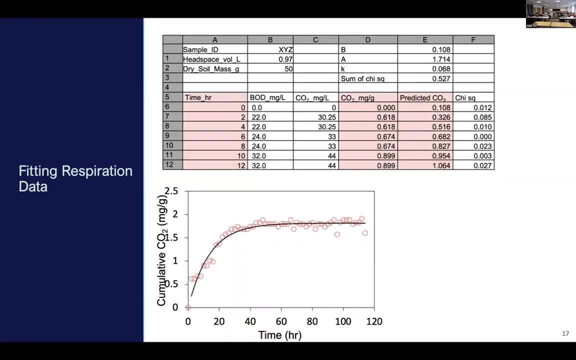 So we can fit our measured data with this equation, such as a good fit like this, So that's kind of tell us those final optimum parameter values. Is this A perfecting And as a comparison on the right? that's the two data points that we collected from one solid soil samples. 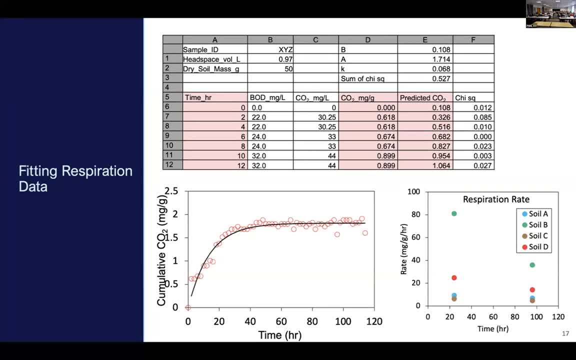 So we can see with this two data points. it's hard to see where the concentration curve off, where we reach to the plateau, But that's the big improvement is this measurement And this data can be further used to elaborate with other biogeochemistry. 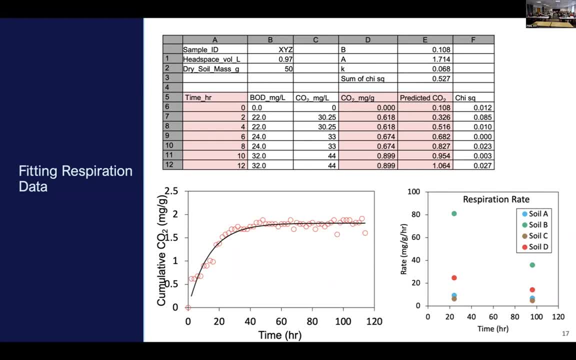 Data, other molecular data for intubation. So I think I set this date up for our tomorrow the hands on learning activity. So we're going to provide you some examples of data, that from Monet. So you can- some of you can- do this fitting by yourself to process this data from draw. 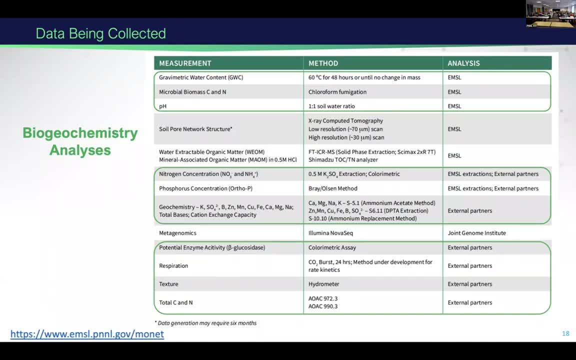 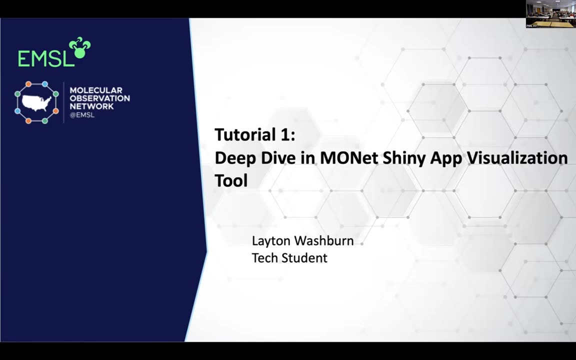 So I covered this respiration on this list. for the rest of those biogeochemistry data, You can learn from latent to how to use our shiny app to explore them. So Layton is presenting online Your turn. Thanks, Jin. Can everybody hear me? 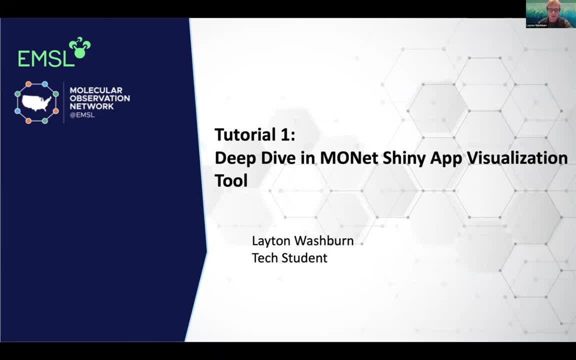 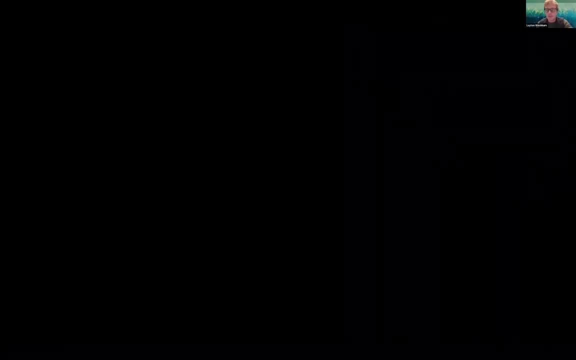 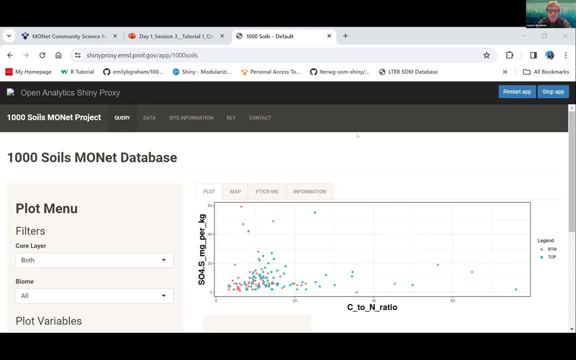 Yes, Yes, Can you hear us? I can. Yes, I do need to share my screen. I think you have to share. Thank you, Can everybody see my screen? Yes, Okay, Well, hi everybody. My name is Layton Washburn and I am a tech student here at PNNL. 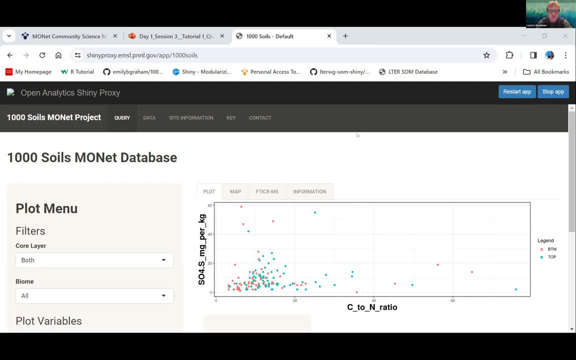 And now we're going to take a deep dive into the Monet shiny application, which is a visualization tool for Monet. This is a. so, first of all, this is a web based application that is publicly available to everyone, meaning that anybody can just go and access the link. 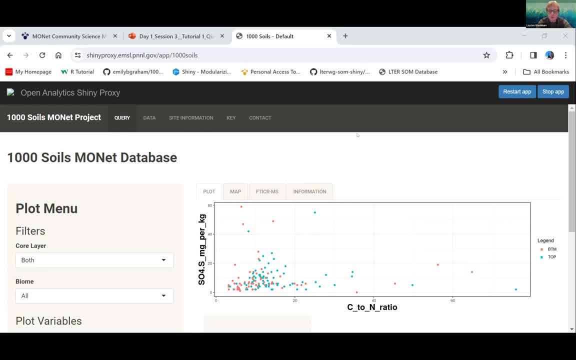 And I believe the link is in the GitHub under this tutorial If you wanted to either follow along or go check that out later. So when you initially? Sorry, I forgot to mention that this is a beta application for a feature, Monet data portal. that was, I believe, talked about earlier in today's session. 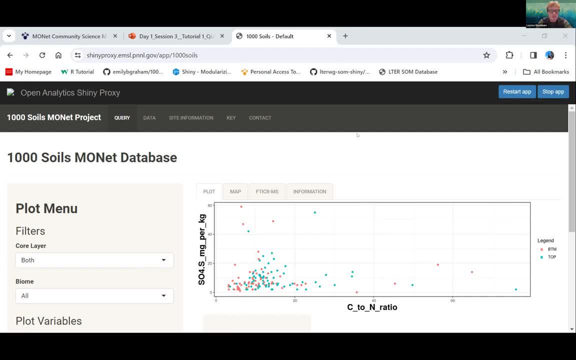 So when you first navigate here, you can see that This is based on five key tabs. So we have our query tab, data site information key and contact tab. Most of the data manipulation and visualizations will happen within the query tab. 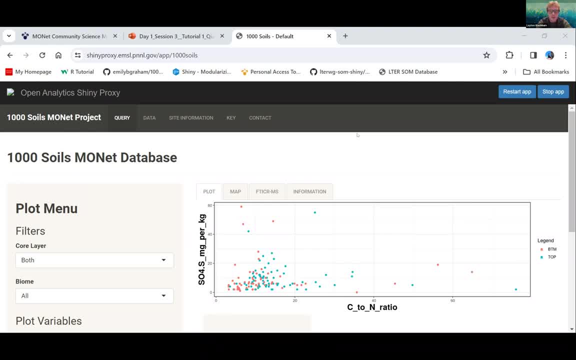 And we do expect most of the users to spend most of their time in that tab. So when you initially start the query tab, it will populate with the defaults, meaning that you will start with a unfiltered data set, And this data is pulled from the bio geo chem data that is found on Zenodo. 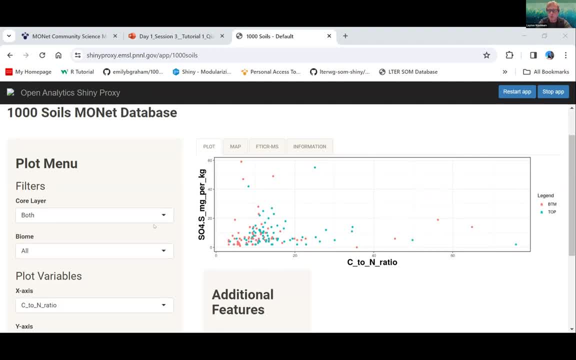 So when we come here, we can see that we have three different sections of our query tab. We have our controls on the left, We have our visualizations on the right with the options of plots, map, FDICR and information, And then we do have a small but powerful additional features section, which I will explain later. 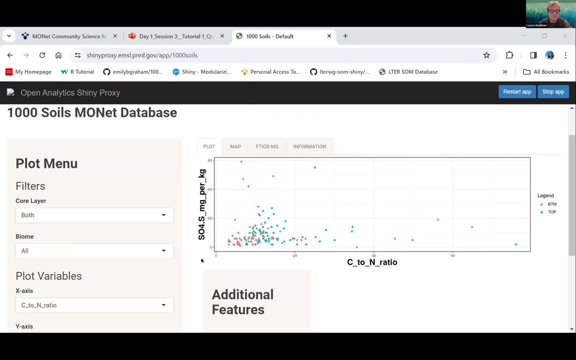 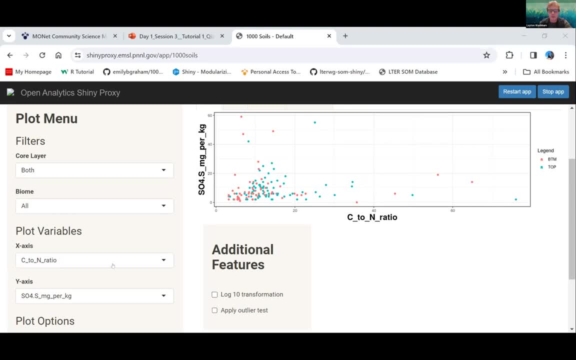 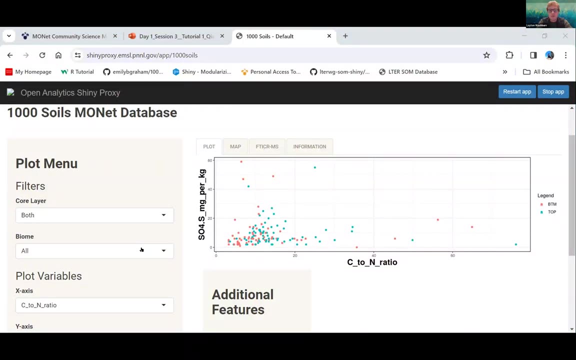 which I will explain later here in a second. so I've gone ahead and I've chosen some data types for us. these will not be the defaults when they load. the defaults, I believe, are the mean GWC, but everything else is the defaults. so when we come in here we have our unfiltered data set and if we wanted for the 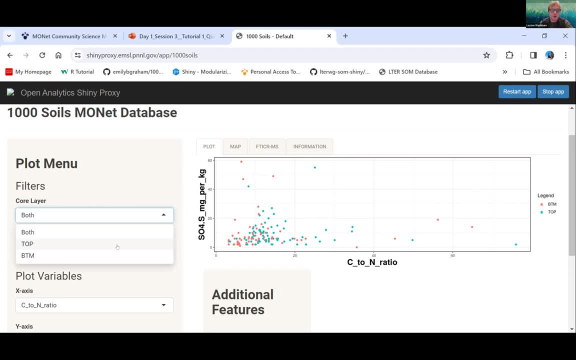 demonstration, I am going to choose a core layer of top, meaning that what this does is it goes through the data set, our data points, and it will select every data point with a core layer of top and then it will apply the other filters, which in this case, is all of the biomes, and then it will 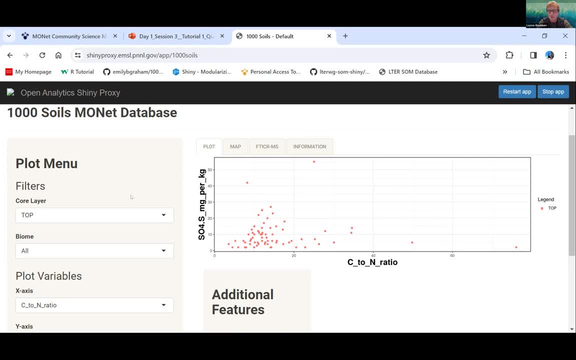 render that to the visualizations on the right. and if we wanted to change biomes, we could. we would just pick one from there and then select it, and then the graph would go through and it would apply that filter to it. so the x and the y axis under the plot variables represent our data types. 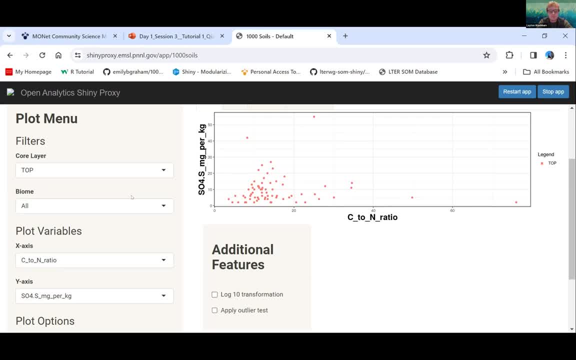 for the biogeochem data set and if you have two specific comparisons you want to make between data types, you just go into there and you plot them where you want, either on the x axis or the y axis. an important note is that, depending on the graph type that you have, either the x axis 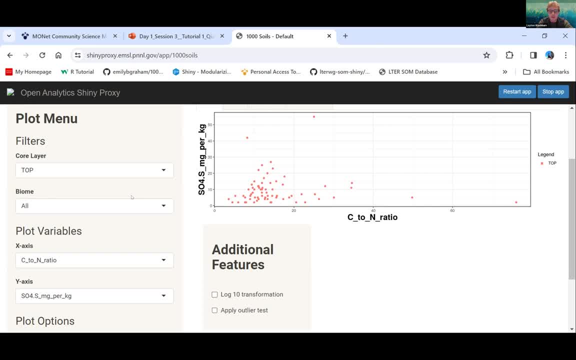 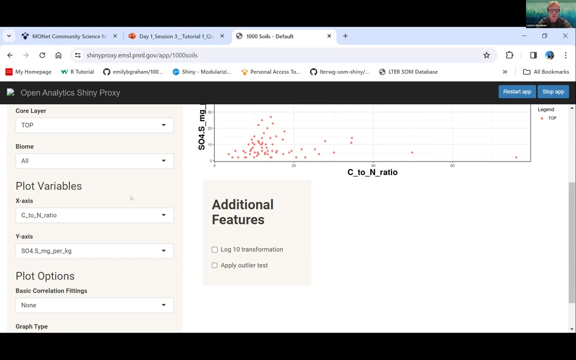 will be the select menu that you need to choose a data type from and the other one will not work. that is a feature we are planning to implement in the future to make that more user-friendly. but after you've filtered for your core layer, your biome, you've chosen the data types that you want. 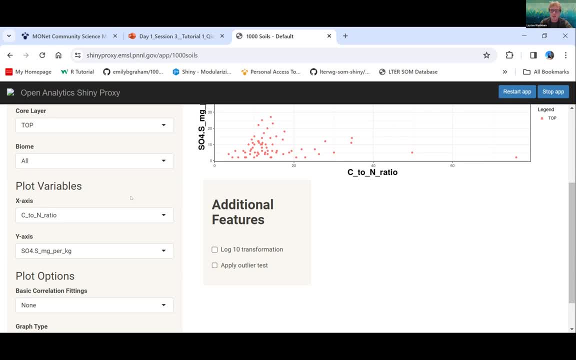 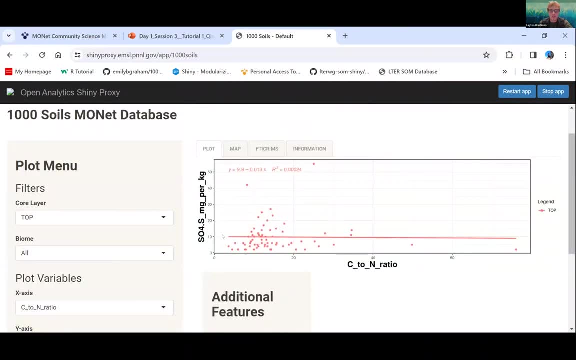 then you can choose. you have the option of applying a correlation fitting, which right now is set to none, but if we wanted a, let's say, linear correlation fitting, we would select that and, as we can see on the graph, that it does apply a linear correlation fitting displaying the equation of the line and the. 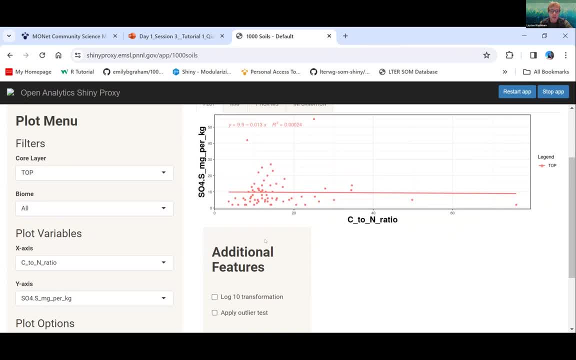 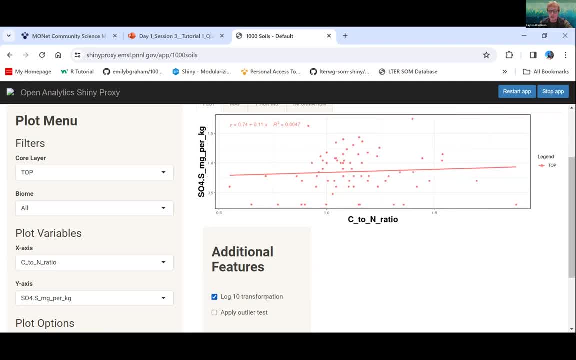 hard to pick apart. we could apply a log 10 transformation and it would make it easier to see for the most part, If we also just wanted to see where most of our data was sitting. we can also apply an outlier test. So when I select that here, it removes all of the outliers. 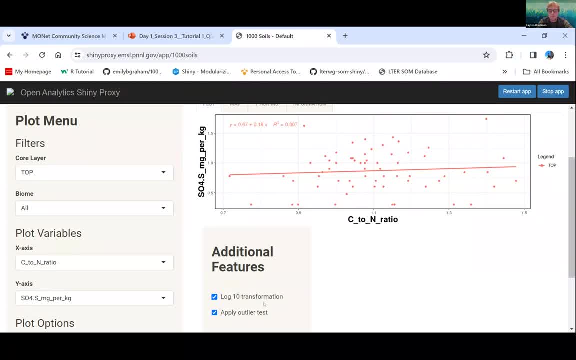 from the currently filtered data set And if you uncheck it, it just does the opposite and it puts the outliers back, And you can do the same with the log 10.. You can undo that And, as you can see, the graph on the right is changing as we are filtering or unfiltering. 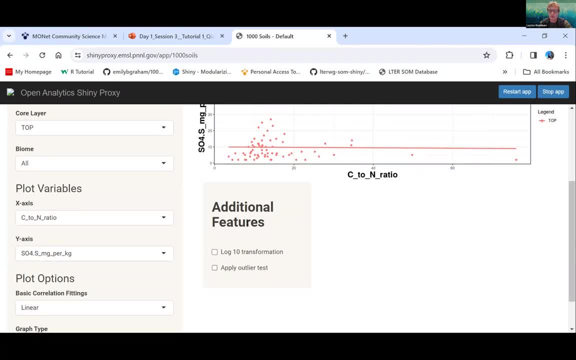 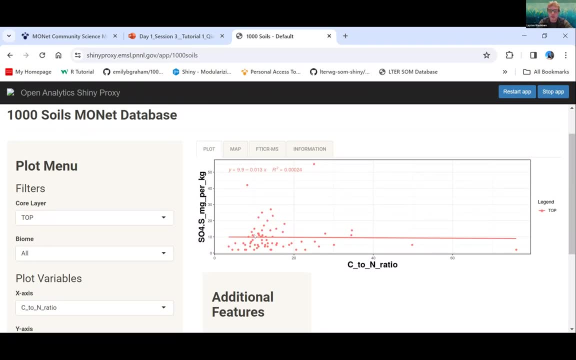 And then you have the option of changing from either scatter plot to a box plot or a histogram, depending on what your goals are for the data and what you're trying to look at. So then, in the visualizations area, we have three more options. 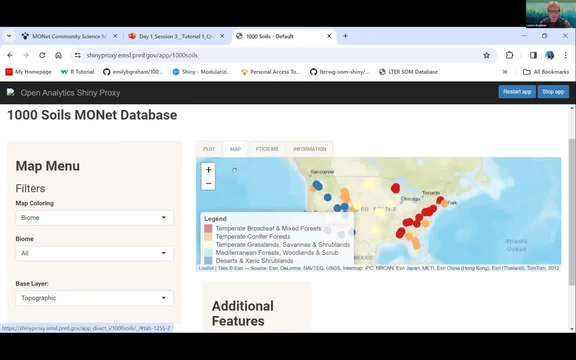 This is map F-T-I-C-R and information. The map portion gives you two distinct areas to look at this data through visualizations. One is the biome and the other is the color variable which represents the data types. This is specifically meant to show the concentration. 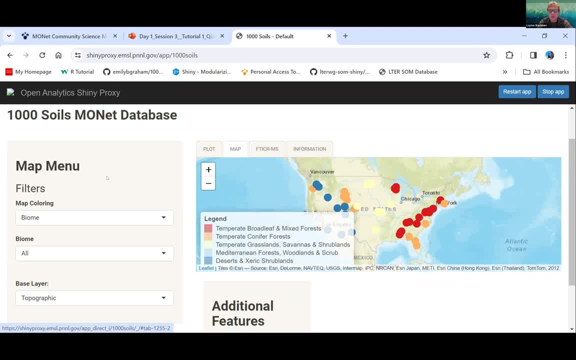 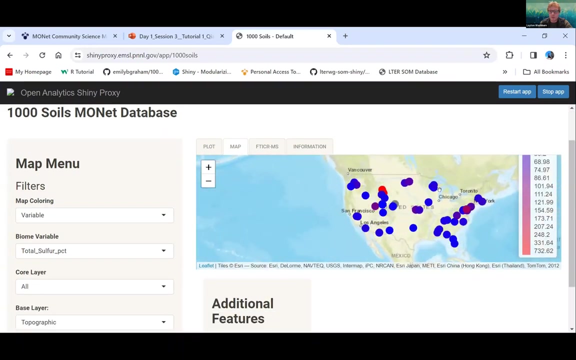 of these, either biomes or the data types. So if we went ahead and chose the variable and we choose- let's choose- total sulfur- we can see the concentrations of this data type- Sorry- On this map here, the blue representing less concentrated and the red representing a. 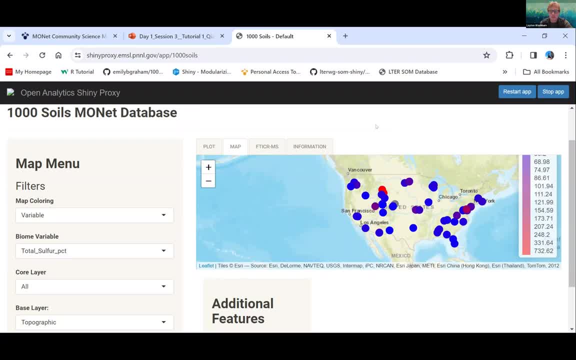 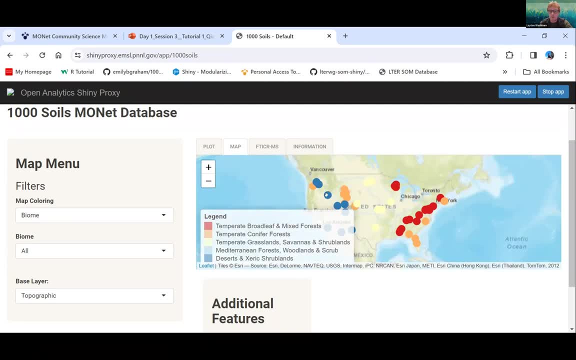 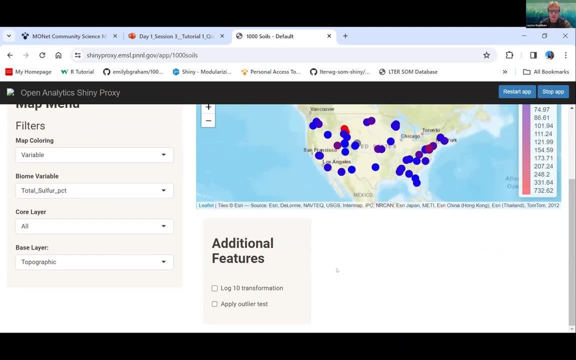 higher concentration in that area. And what is nice is, if you want to go back to biomes, you can also see where those are relative to other biomes, Kind of where they are in different areas. So we also have the similar additional features tab where you can apply an outlier test and it. 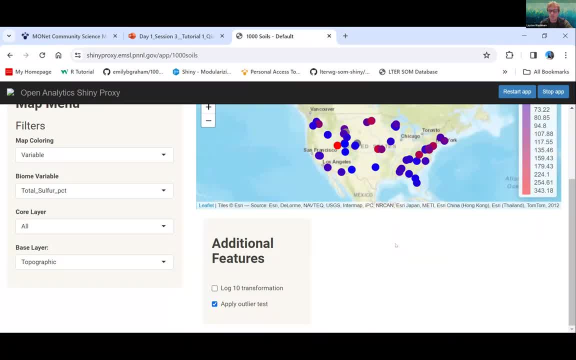 removes that from the set that you are filtering for. So if you didn't want to see where your outliers were in regards to the continuous scale, you just apply that and it will remove it and it will render everything accordingly. It will take it out and it will be able to see where your outliers 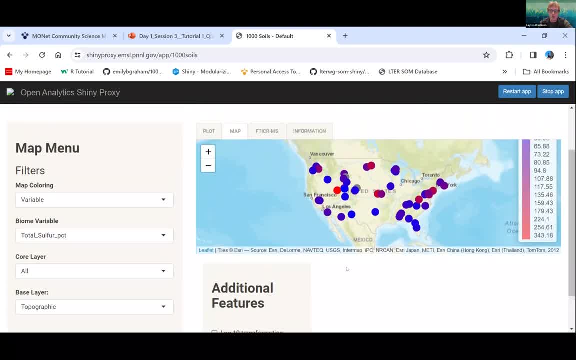 are and recolor everything as needed. We also have the Core Layer filtering option here, meaning that if you wanted to look at a specific core level, like top or bottom, you could go in here and you could filter for that And it would render it to that changing the scale also, And then you can change the base layer, if that's. easier, or if you have a preference on the base layer here. So then we have our FTI CR and it's a DHS. you can go in here and change the base layer. But if you have a preference on that, there's a. 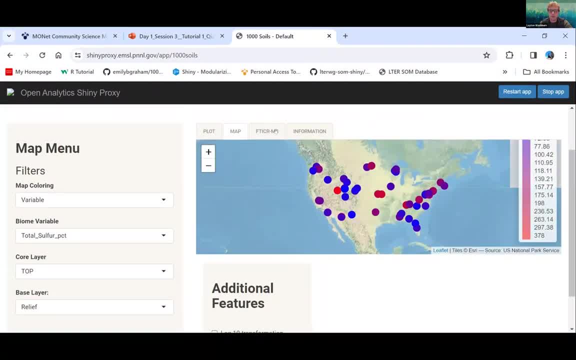 base layer here And then you have the base layer. If you have a preference on that, the base layer here. So it's nice to see something in the middle here and it's really helpful. but you can use it to the lower integrated field. you can use that, But you can get it in these other layers as well And we 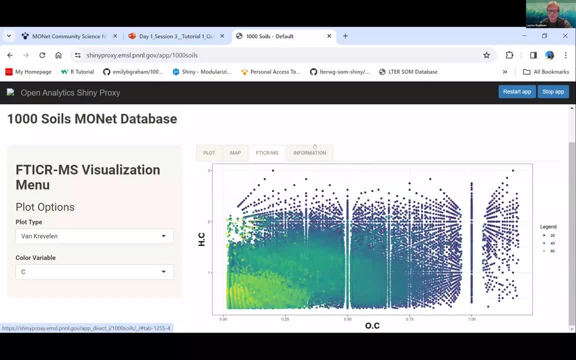 And a quick note about that is: this will be talked about in a later tutorial today by, I believe, Will and Nicole. Correct me if I'm wrong on that, though, but I think that's the FTICR. But when you initially come to this tab, we start out with our event prevalence, and then it sets to a default of C for the color variable. 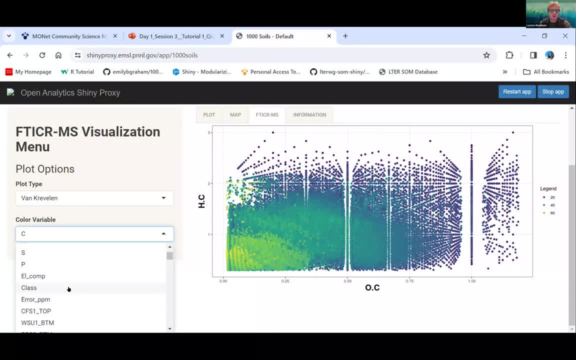 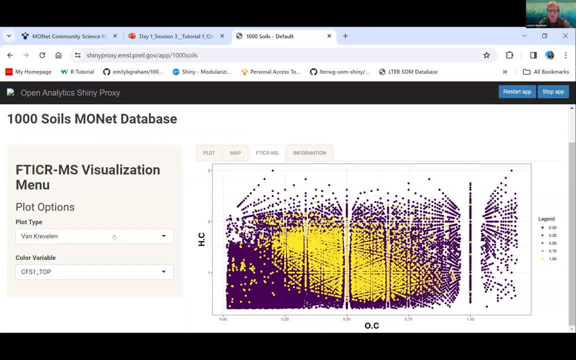 And I think an easy way to see this is if we go down to a specific sample. What this means here is: on the right you can see the legend, the purple being peak absence and the yellow being peak present, And our data is just zero and ones for the peaks present and absent. 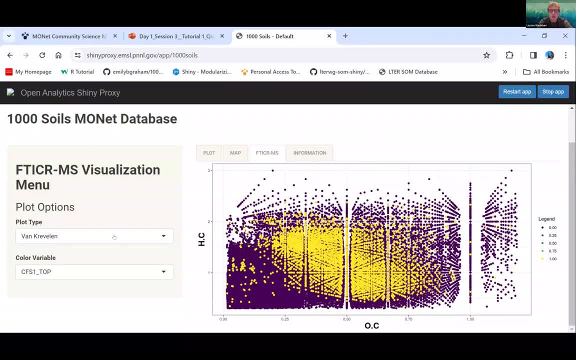 So we won't have any of those in between colors. But as you can see here we have for this specific sample, CFS one the top- we have a specific set of peaks present. So if we compare that to another sample, 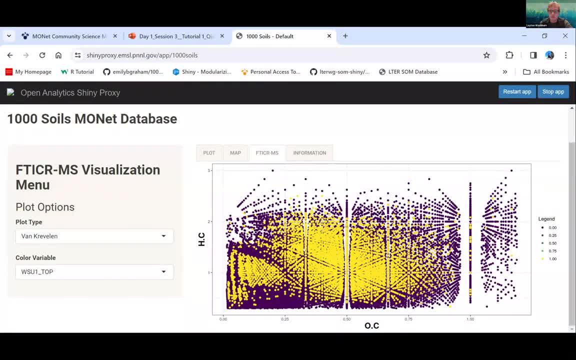 let's just choose another one. We can see that the peaks present changes in different areas, which shows us that each of these samples has a different composition, So it is nice to be able to come in here and to be able to quickly compare samples and to be able to 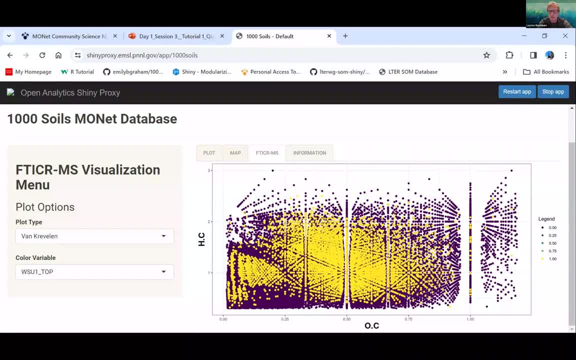 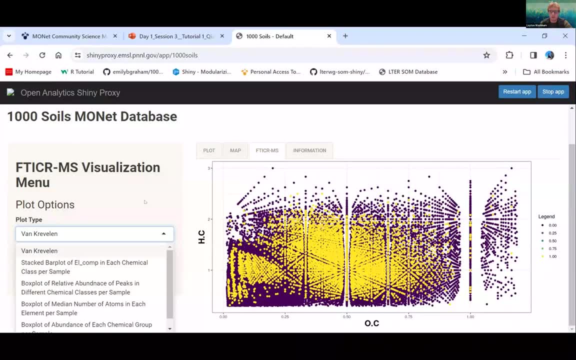 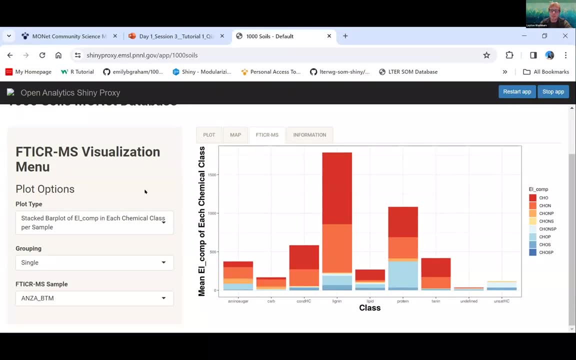 be able to really like manipulate the data and to see that You also have a couple of different options for the plot type in the FTI-CR. You have a stacked bar plot which provides a single sample and a multi-sample comparison plot. 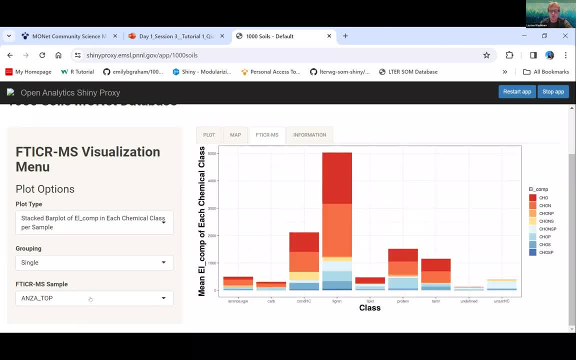 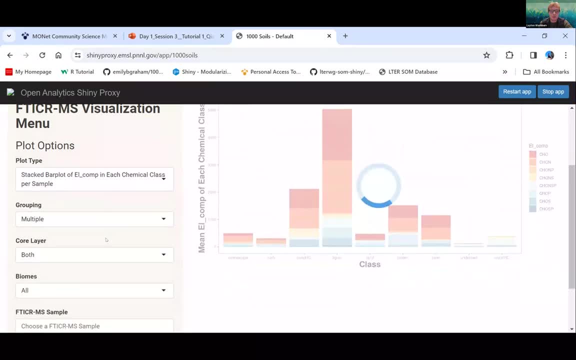 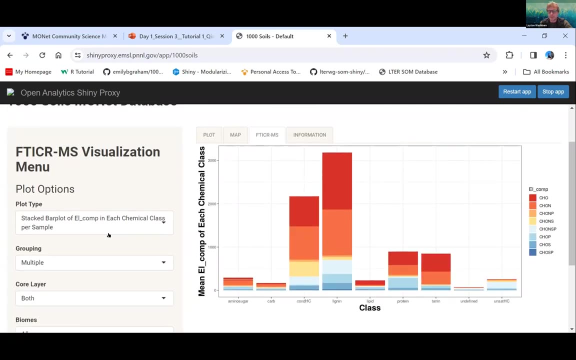 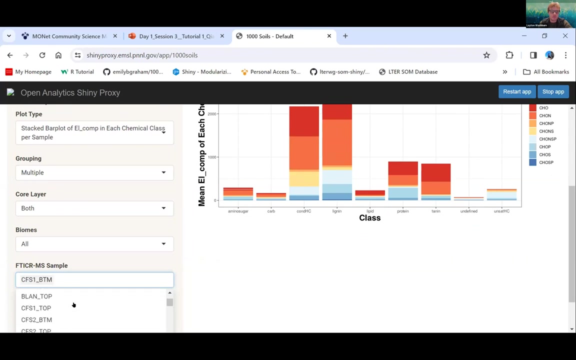 You can filter by sample and you can choose the specific sample you want and the graph will render to that sample. Or you can have the option of comparing multiple samples all at once. It does take a second to load as a heads up. So let's say we wanted two samples. The graph would apply those two samples and put them on the plots here. 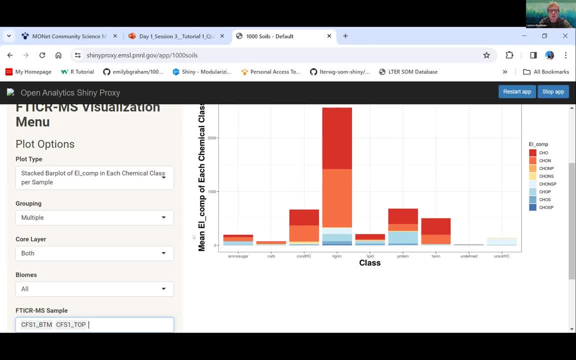 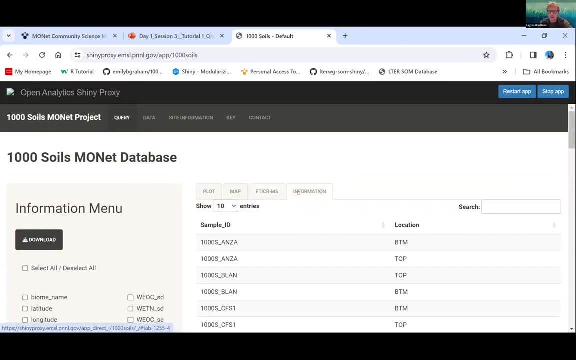 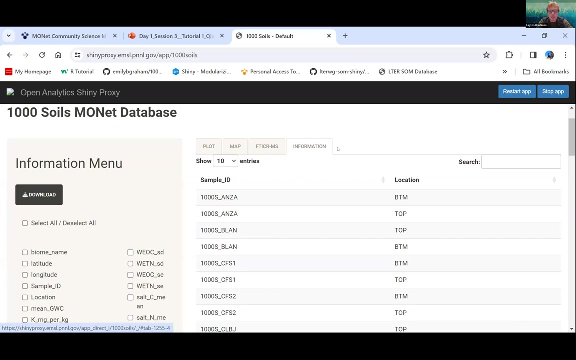 And you also have the options to filter for the biomes and the core layer as well, if you wanted to. So let's set the data from there. And finally, on our visualization area, for the query tab, we have our information, And this is just meant as a quick way to download the data. 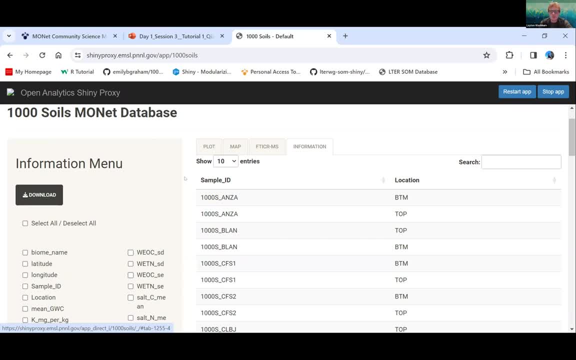 So you can select either all of the data- And these options here on the left are the data types in the biogeochem data- And you can select the ones that you want And it will show you what you have selected on the right through a data table. 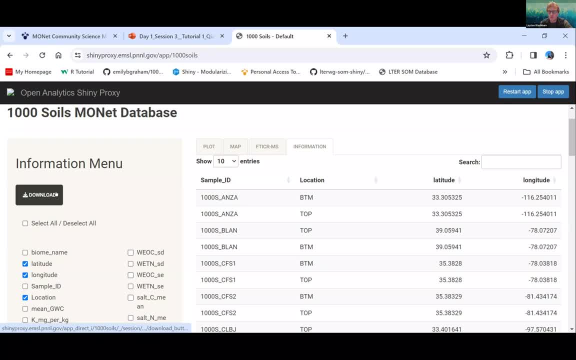 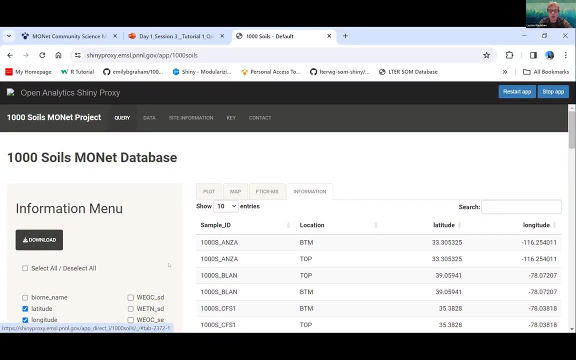 And then you can download that, And I believe it is the CSV that it downloads for you The data. So, moving on from here, now that we've explored most of the visualizations area, we're going to take a look at the tabs that are meant to provide context and to provide metadata for this application. 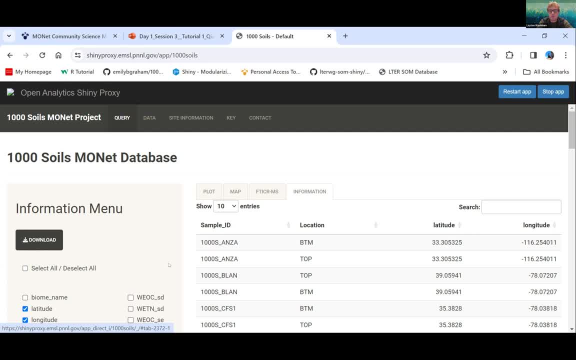 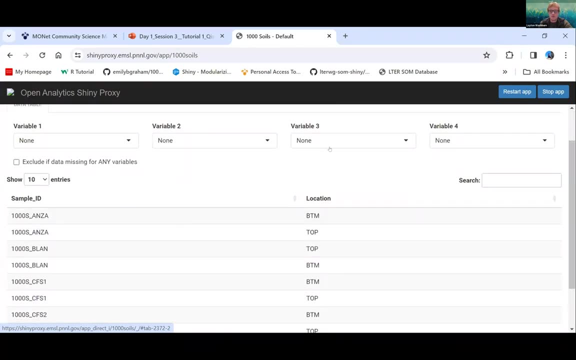 Just keep in mind that the query tab is where a majority of the time will be selected, Just because that's where all the visualizations, or a majority of them, are located. So here we have a data table and this is the data tab, And you can choose up to four variables. 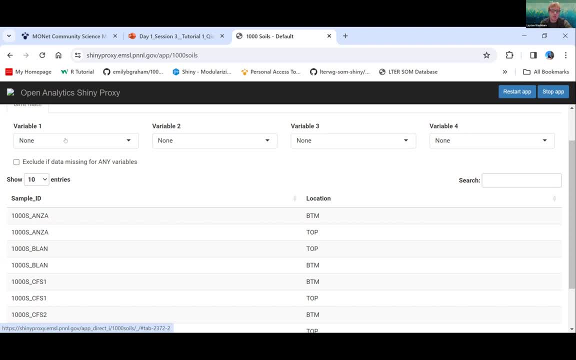 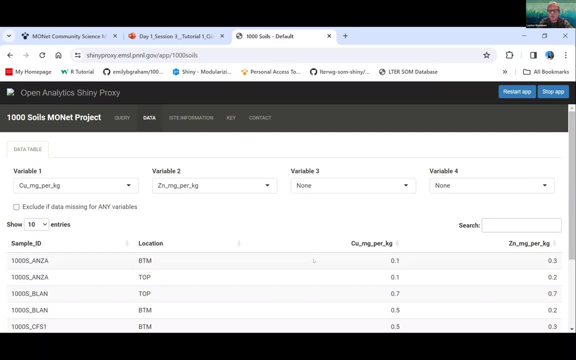 You don't have to choose all of them for this to render, So if I just choose a couple of random ones, we can see that the data table below adds those to the right on the table, And it's just a quick way to be able to look at the numbers. 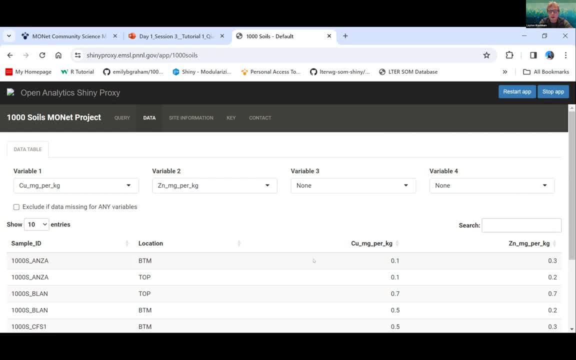 Or the data there without having to see it in a plot. So it's more of just being able to see the numbers directly or to be able to see more of like the raw data from that And you can choose up to four variables And you also have a checkbox to exclude data if any variable is missing. 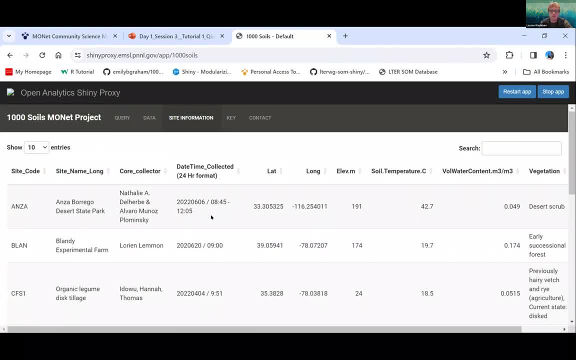 The site information is primarily meant to provide context on the sites Such as, like the core collector, the date and time it was collected, the latitude, the longitude, the elevation and so on, And it's just in another data table format. 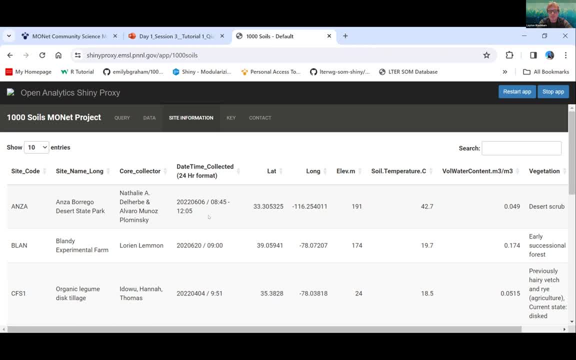 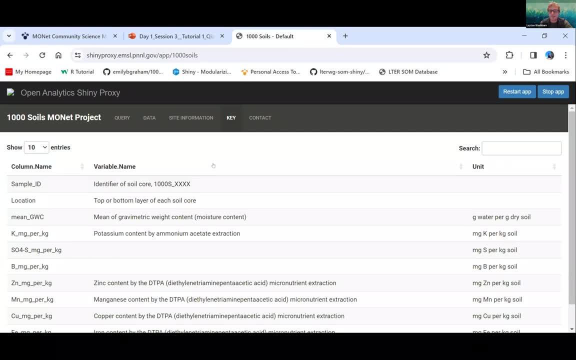 So you can quickly see the numbers and just navigate to a specific site if you want to. And finally, our key tab provides context on the data, types, variable names and the units that it was collected for. So if you were wondering specifically what units it was or what the variable name was, 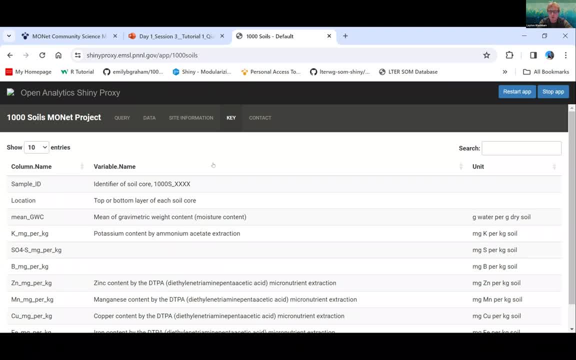 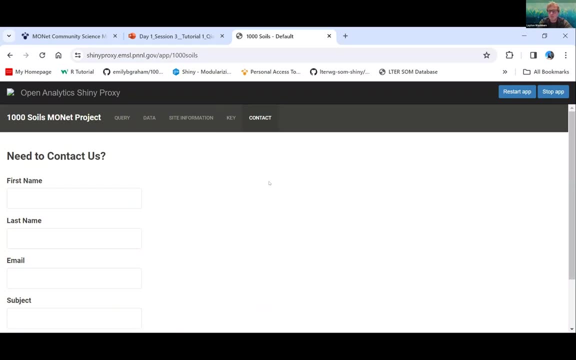 you could come here and quickly search for the data type that you're comparing. So that is a majority or that is a dive into the MONAT Shiny application. If you have any feedback, suggestions or if you find a bug, you can come over to the contact tab. 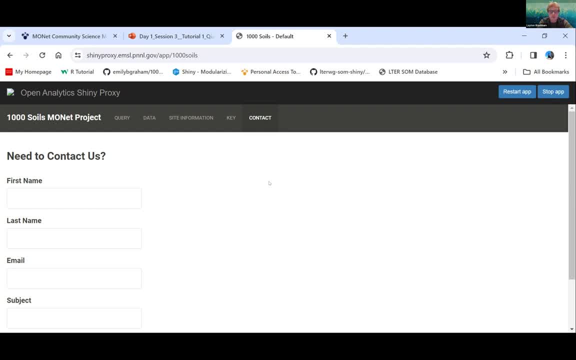 And you can fill out the text fields And then submit it And it will be sent to a monitored MONAT email And we will get back with you soon. And now Kaizad will be. I am going to hand this over to Kaizad. 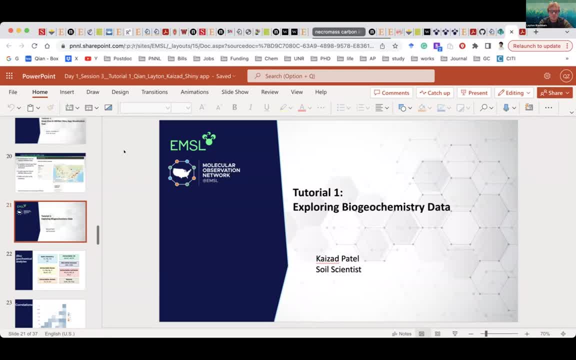 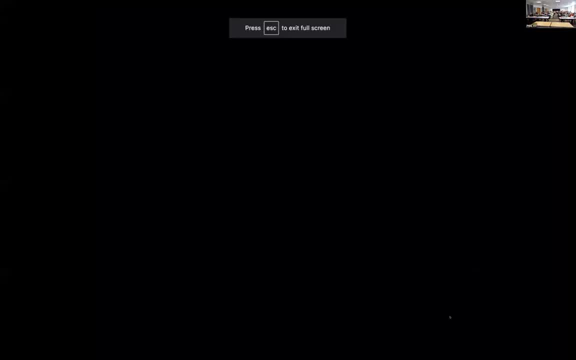 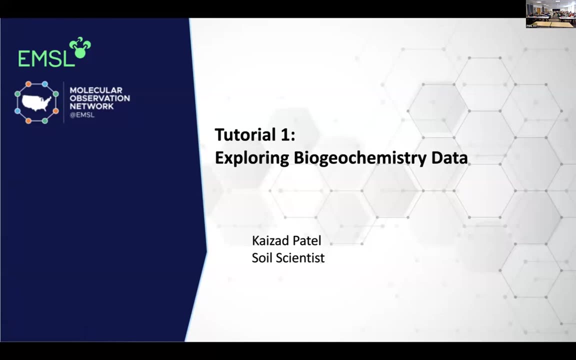 Kaizad Patel. I'm a soil scientist at PNNL. Today I'm going to talk about some of the data that we've processed and we've analyzed, And this is basically a very preliminary look at the data we've got. This will be a complement to what Layden just showed us. 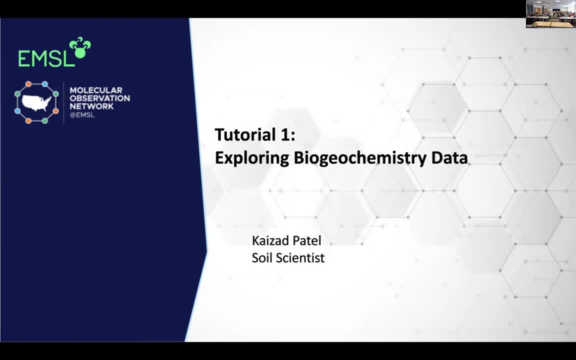 So he showed you how to work through the Shiny app. I'll show you some examples with the Shiny app, along with some outputs from R And a lot of this just a heads up. a lot of this is basically like soil science 101.. 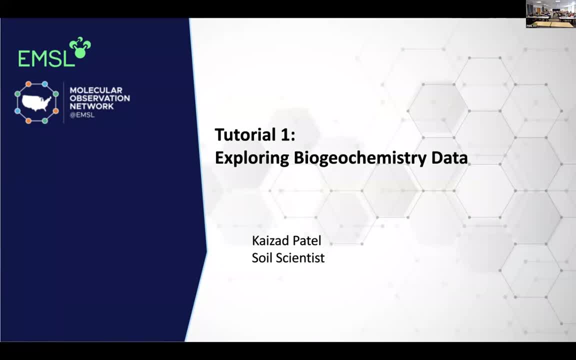 So you might say, oh, carbon and nitrogen are correlated. Wow, what a big shock. But this is just showing you. you know, initial glance at our data And we're still doing QAQC. So like what do we look at to make sure our data are good? 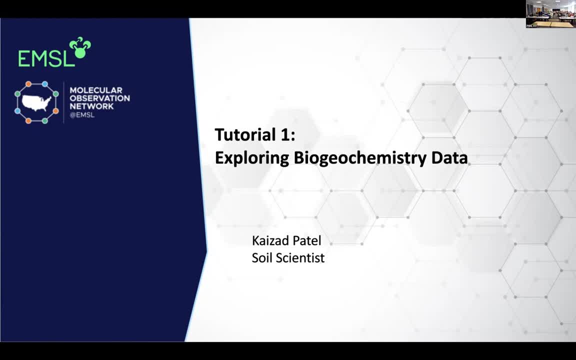 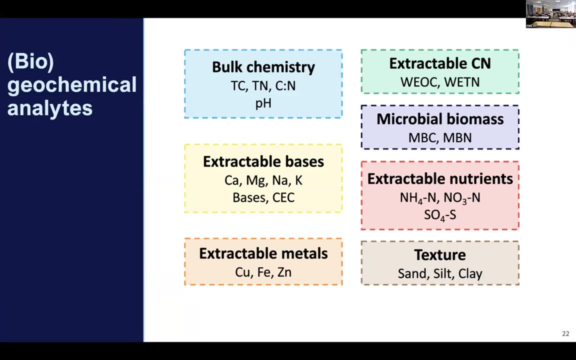 That's basically what I'm going to show you And, of course, we'll have our hands-on tutorial session tomorrow where we can dive deeper into some of these correlations, some of these variables, and we can answer specific questions. This is just like a high-level overview of what's going on. 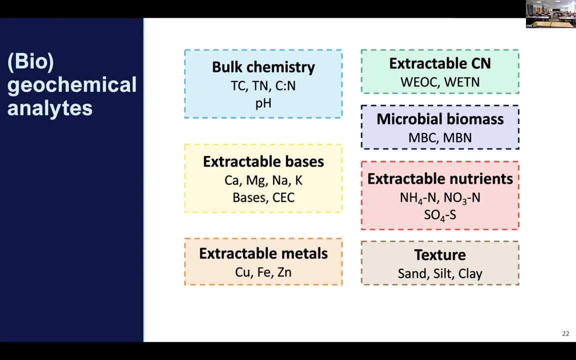 OK, So, as Jen mentioned, we've got a bunch of analytes that we've been measuring. I've broken these up into different groups So you can see. we've got bulk soil chemistry like carbon nitrogen and pH. We've got some extractable variables. 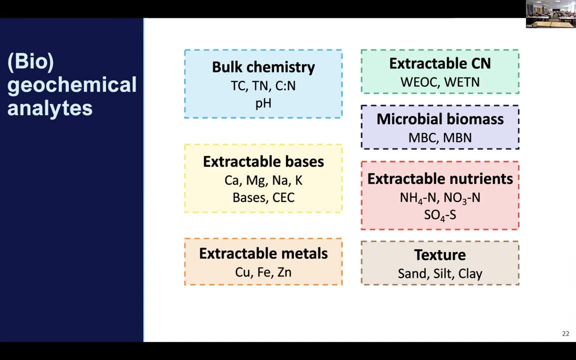 So water, extractable carbon and nitrogen. on the top right, Microbial biomass. We've got some geochemistry going on And then finally we also got some soil texture. And again, this is a small subset For the MONAT samples that are coming up. we have even more analyses coming up. 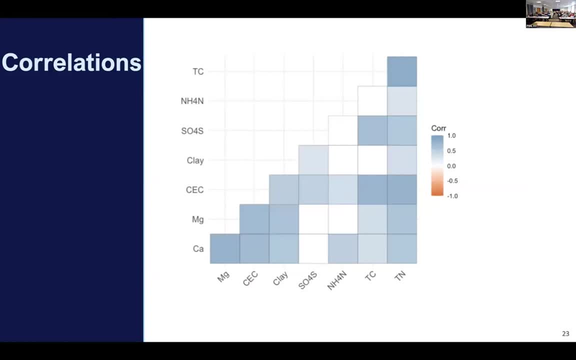 OK, So LATED showed you some correlations using the Shiny app, And the Shiny app is great. if you don't know R, or if you don't want to spend the time coding stuff, or you don't want to work with Excel, That's great. 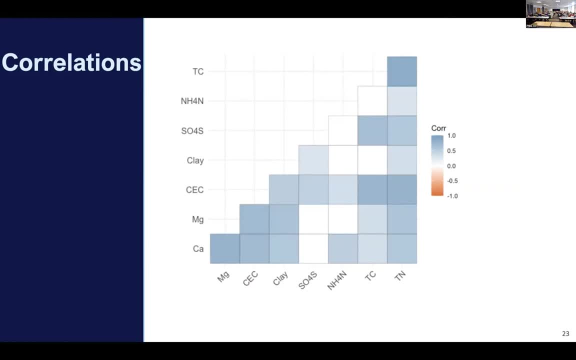 But that's good for like one-to-one correlations. What if you want to put everything in one big matrix and want to look at trends overall? That's what I've done here using R, And this is just. I've just pulled out six or seven variables because you know, if you try to look at all of them all at once, it's just a lot of stuff. 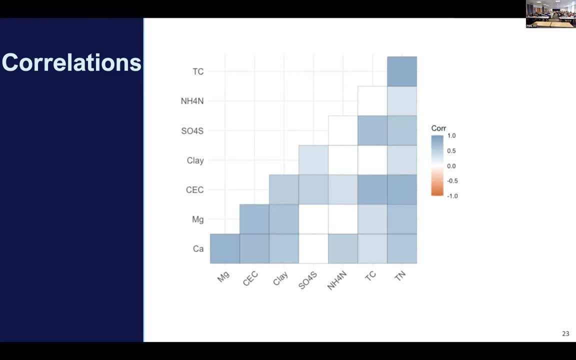 So here we see the correlation matrix for variables that were significantly correlated, And everything on here is shades of blue, which means everything is positively correlated, And a lighter shade means it's less strongly correlated. The darker the shade of blue means it's more strongly correlated. 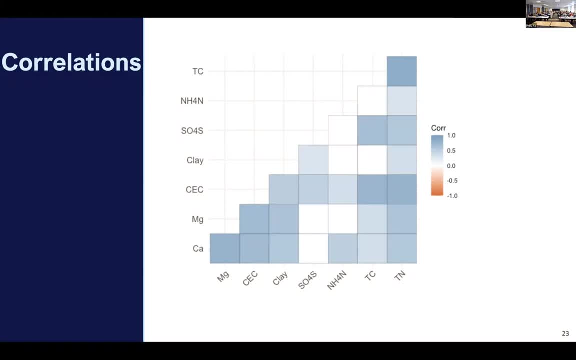 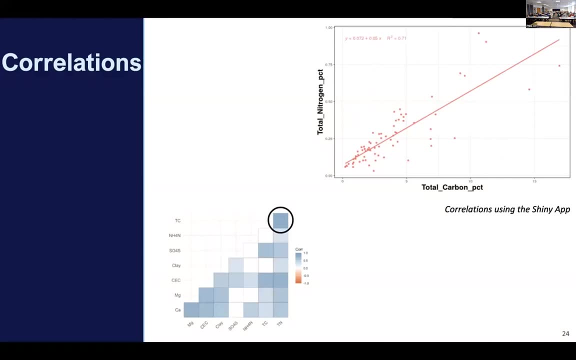 You can see, there are some things here that are correlated, and I'll show you some of those. The first one is total carbon: Total carbon and total nitrogen, As I mentioned. no surprise those are strongly correlated because the carbon and nitrogen cycles are quite closely linked in soils. 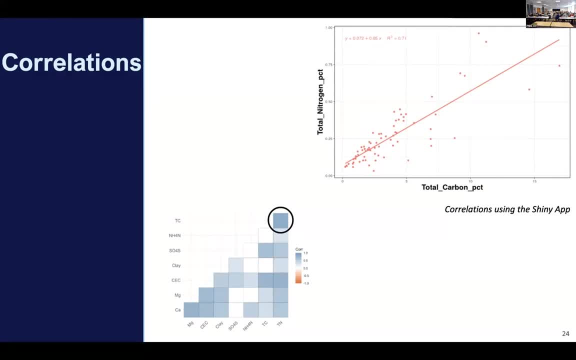 That's to be expected, But again, this is just one of those things to make sure. Just one of those things to make sure our data look good, right If something's super wonky. that's our first metric, And I want to point out this top graph that I got using the Shiny app. 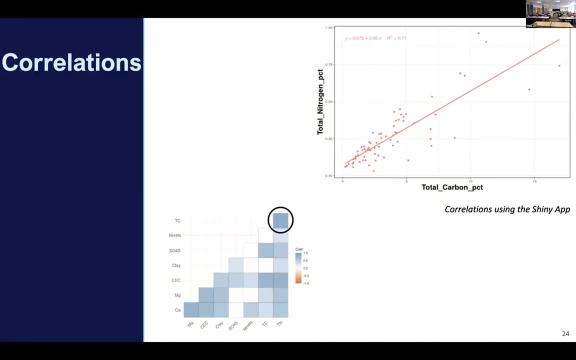 The one on the bottom left is using R. So of course different methods, but they still work together. Total carbon was highly correlated with many of the variables. I guess that's to be expected. So here we've got extractable sulfate, which is a nutrient. 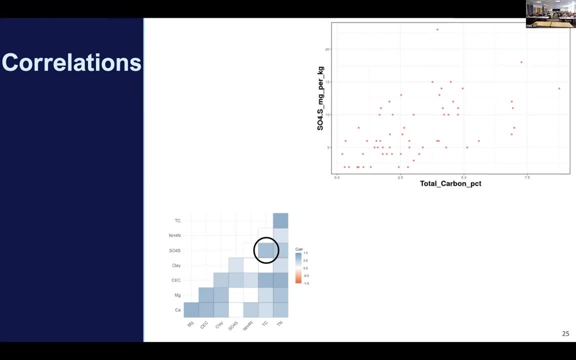 It's also a terminal electron, It's an electron acceptor, So it has redox- redox connotations as well. Quite strongly correlated. Total carbon and CEC, that's cation exchange capacity, So it's the capacity of the soil to hold on to cations. 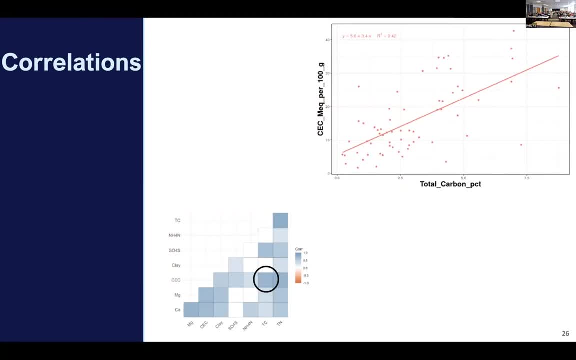 Basically it's a measure of the negative charge of the soil And that's correlated with total carbon. If we assume that a lot of our carbon is organic in nature, that means there's a lot of negative charges in our soil. That also means we would have high CEC. 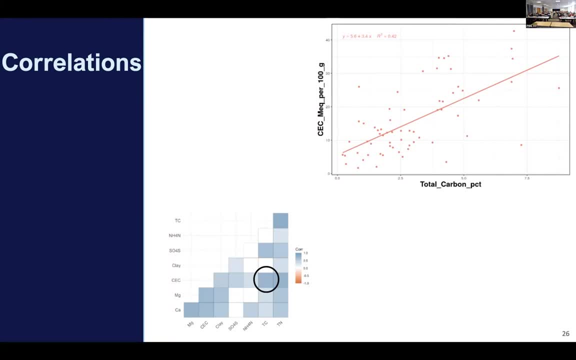 And I'll show you some maps later where you can see those relationships. So, again, not surprising, but it's good that we see those correlations. CEC is also correlated with clay And again I want to point out this is preliminary correlations. 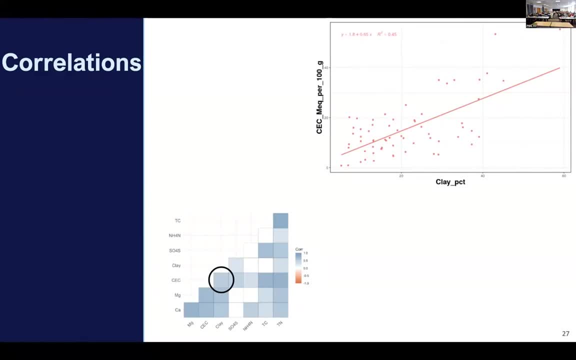 Correlation does not equate causation, So just take that with a grain of salt. This is what we see from our very limited database. As we start pulling in more samples, we might start seeing different trends, right. Different trends in different biomes, different trends for top horizon versus bottom horizon. 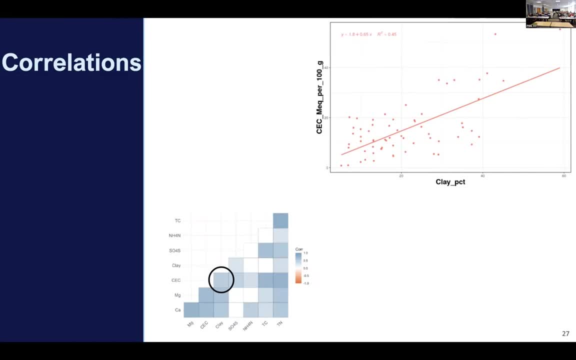 Some different trends might like show up Here. we've got CEC versus clay And again, the more clay you've got, you're going to have higher surface area. You're going to have more negative charge, which again would correlate to more CEC. 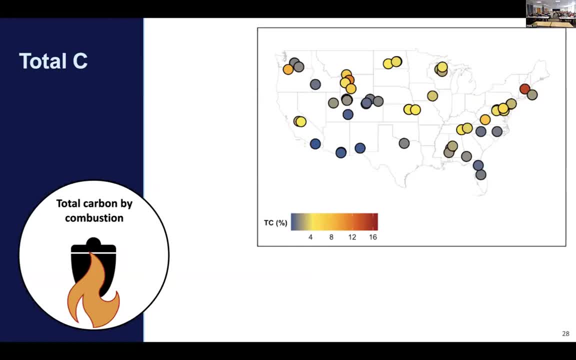 All right, Now I have some maps here that will show you a graph, And we're going to take a greater dive into some of our variables. The first one is total carbon And, as Jen mentioned, we measure total carbon by combustion. 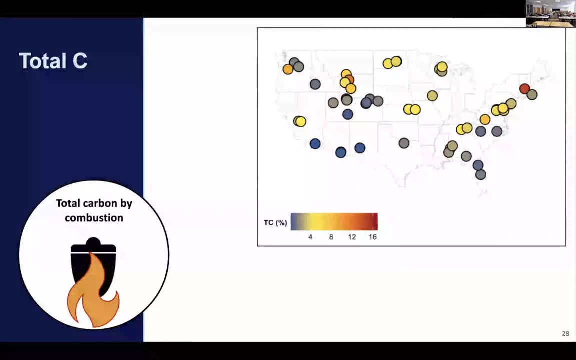 We take our dry samples, We heat them in the presence of oxygen at about 900 Celsius. So we're basically converting all of our carbon into CO2, all of our nitrogen into gas, and we measure that And we do some math and we get back to total carbon percentages. 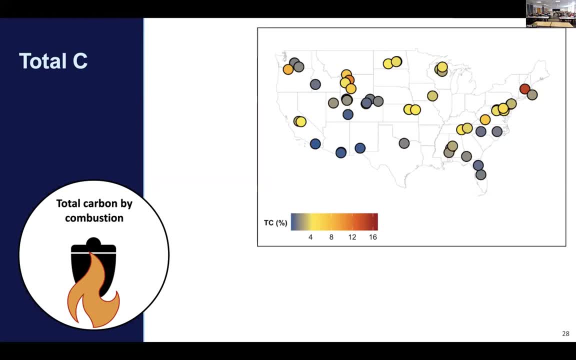 This map here. this was done in R, So it's a different version compared to what Leighton showed us, but the same data. So we see a wide range in our total carbon concentrations, going from about 0.5% all the way to about 16% or 17%. 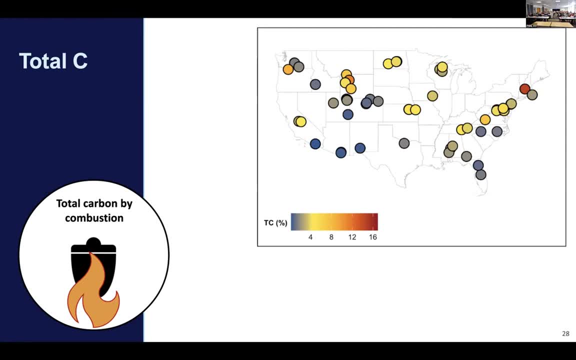 Most of our data are less than 4.. But as we see, up here in the top right, Massachusetts, we've got something that's really high. The Midwest is, you know, medium carbon, So we've got those things going on. 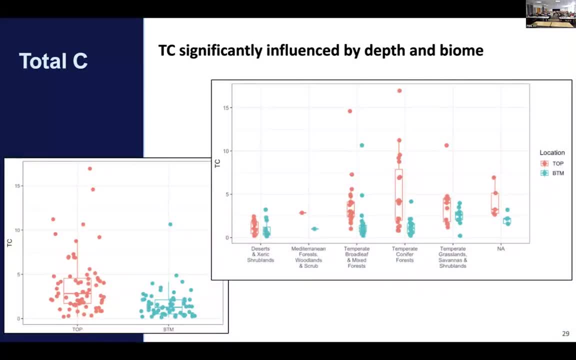 And you might wonder. we've got things like depth, We've got things like biomes built into our data set. How did those influence carbon concentrations? What were the drivers of carbon? We ran ANOVAs, the analysis of variances, very simple stats in R. 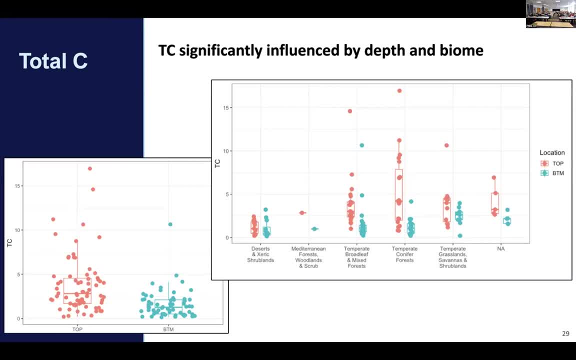 And we found that total carbon was significantly influenced by depth and by biome. So this graph here on the left, that's total carbon split up by the depth. So we've got the top depth in red, because the bottom depth in blue And, as we expect, the top soils have more carbon than the bottom. 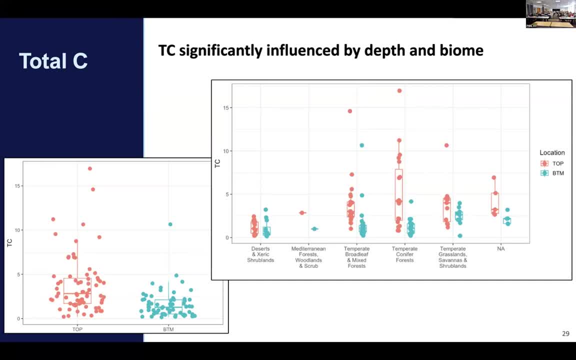 Not a surprise, but it's just good, because soils don't always cooperate with you, So it's just good to see these things actually work as expected. Strong correlation here, Strong differences. The next one: we've got the biomes, And again biome was a strong driver of total carbon. 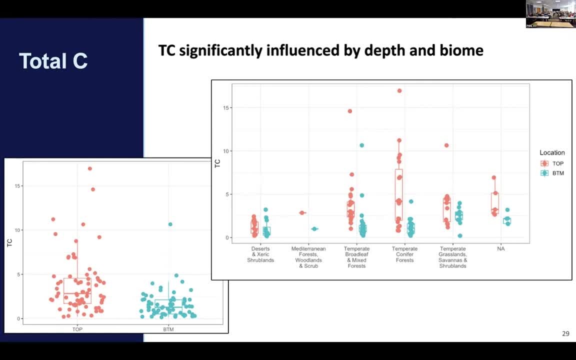 And, as you can see, here there's a lot going on. But again, the top is denoted in red, The bottom is denoted in blue And here in the middle we've got the temperate zones. These were highly variable, but also highest carbon values. 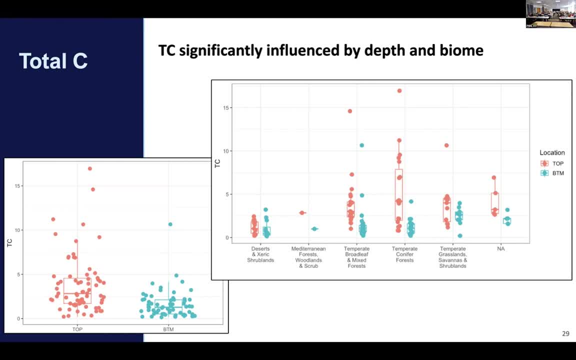 But as here, the one on the left, that's the desert And, as expected, lowest carbon values. That tells us, yes, we've got a biome influence Deserts. there's less vegetative input, so there's going to be less carbon in our soils. 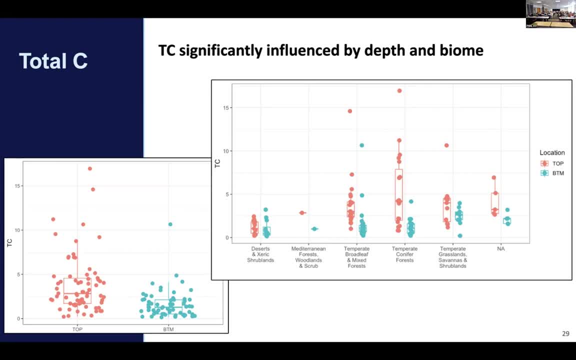 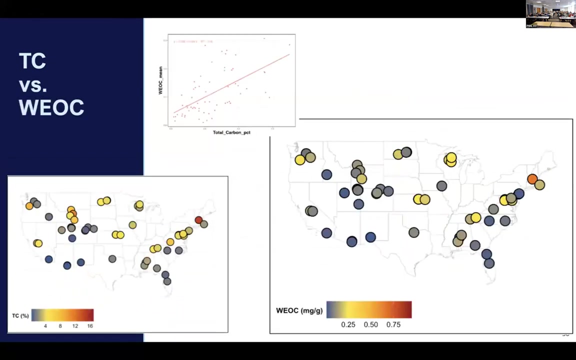 The temperate zone. we've got more plant input, We've got conifer needles coming into the soil. With slightly colder temperatures there's going to be less decomposition, so more carbon accumulation in our soils. All of that makes sense. And again, if you're interested in specific sites, we can pull out certain biomes. look specifically at what's going on within a biome at different sites. 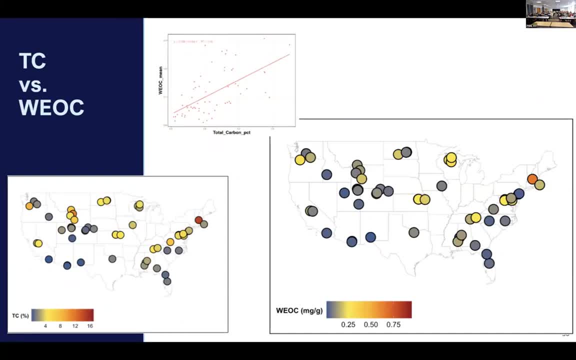 Another thing we looked at was WEOC, which is water extractable organic carbon, And that's one of the fractions of carbon in our soil. So total carbon represents the entire mass of carbon in our soils And you can split that up into different types. 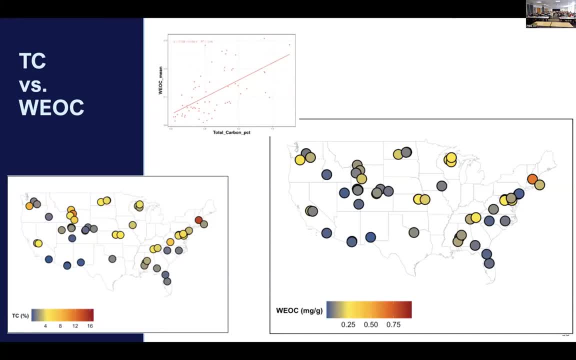 And, as Chen mentioned, we've got water extractable carbon. We also have mineral-associated carbon. Water extractable represents the bioavailable or the labile form of carbon. Basically, what we're doing is we're taking soil, adding water, shaking it, filtering it and then measuring that. 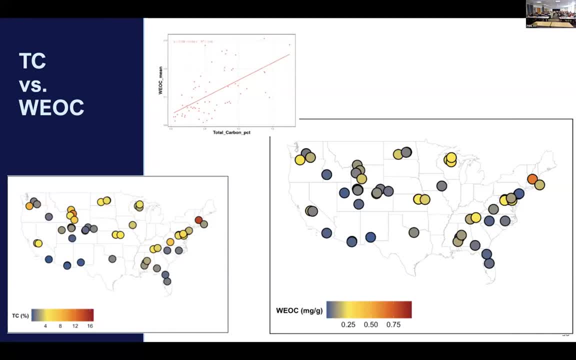 So that tells us what's available to the microbes for consumption And, as you might expect, total carbon and water extractable carbon should be correlated, And that's what we see here. This was done using the Shiny app And if you look at the maps- the geographic distribution- of course there's going to be something. 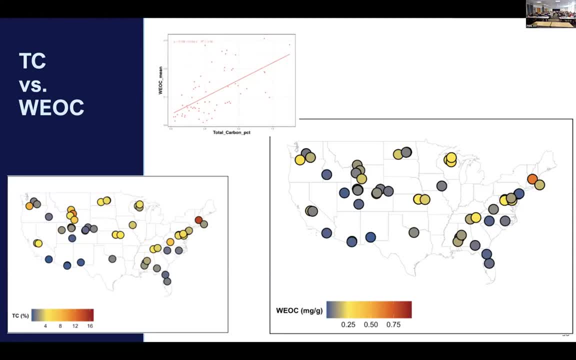 There's going to be some differences between total and water extractable, But overall the trends are similar And, especially if you look at some of these high values, The high value in Massachusetts translates to a high water extractable carbon, even in the same site. 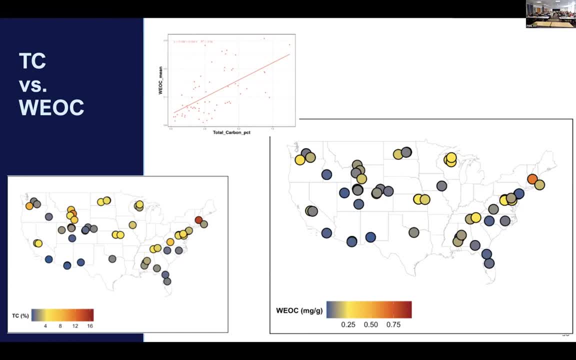 So at least in that sense it makes sense to us And of course for this round, for the 1,000 soils, we did not do mineral-associated organic matter, But that's something that's coming up in the next round. 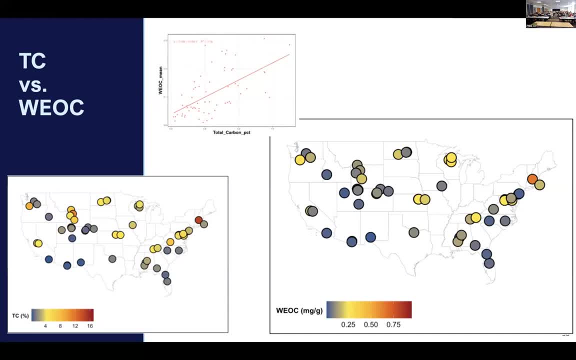 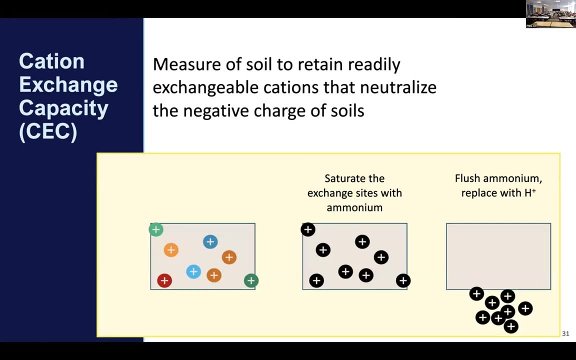 And we're really excited to see how these different fractions work. Next, we have cation exchange capacity And, as we've talked about a little bit today, it's the measure of the soil to retain cations, And that's important because cation exchange capacity tells us how strongly or how much the soil can hold on to nutrients. 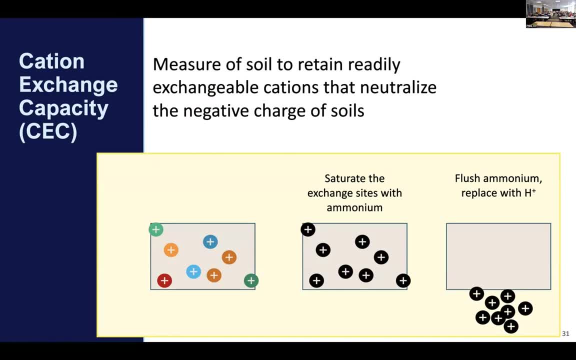 It's a measure of the capacity to release nutrients into the soil. Basically, if you've got a higher cation exchange capacity, you'd have more calcium, you'd have more magnesium And also a higher chance of having more nutrients like ammonium in your soil. 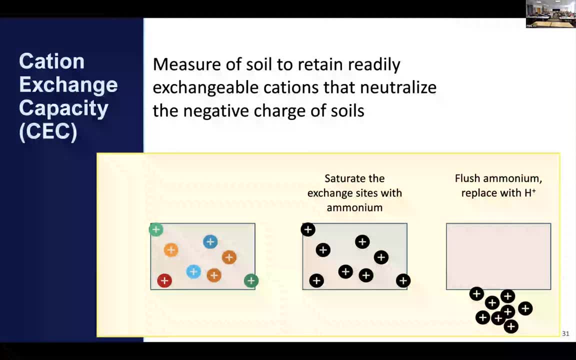 And of course it's correlated with many other variables. But the way we measured it here was we used the ammonium exchange method, Where here we've got our original soil representing the different cations in here We saturate the exchange sites with ammonium. 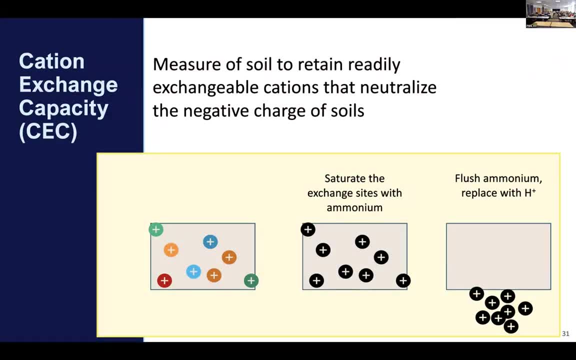 So we're taking ammonium acetate, shaking it with our soil, So all of the cations are removed from the soil surface, Replaced by ammonium, Then we drain the ammonium out, So there's only the ammonium that's left on the surface. 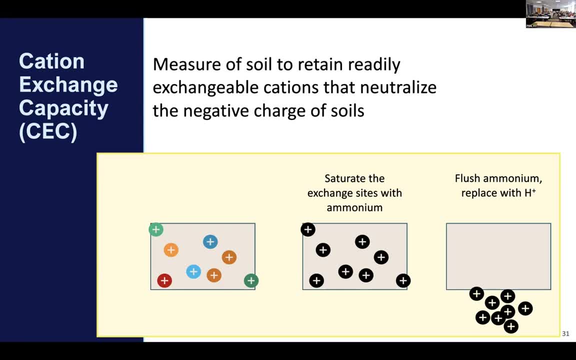 There's no extra stuff left, We add hydrochloric acid, shake it again. So now that exchanges with the ammonium, And then we measure the ammonium that's released. So in that sense the ammonium that we're measuring represents all of the exchange surfaces on our soil. 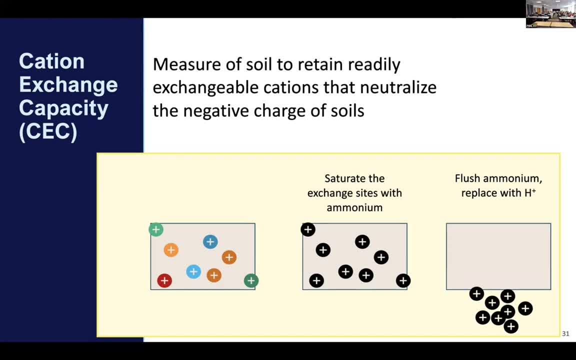 And because these are cations. cations would bind to a negative surface, The This is also a good measure of the negative charges on our soil surface. So basically, the more clays you have, the more organic matter you have, The higher chance of negative charges on your surface. 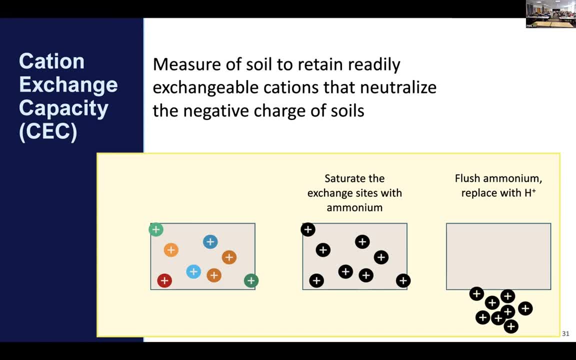 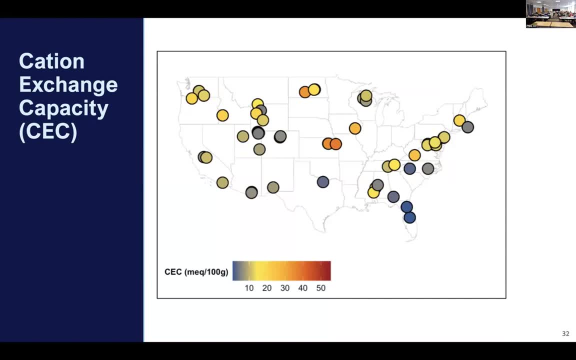 So you have a higher CEC as well. And just a quick 101 for CEC. All right, And we see some interesting trends here. The Midwest especially has high CEC. So if we were to look at a map of clay, maybe 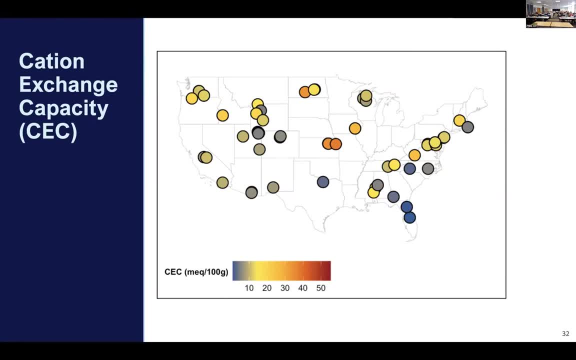 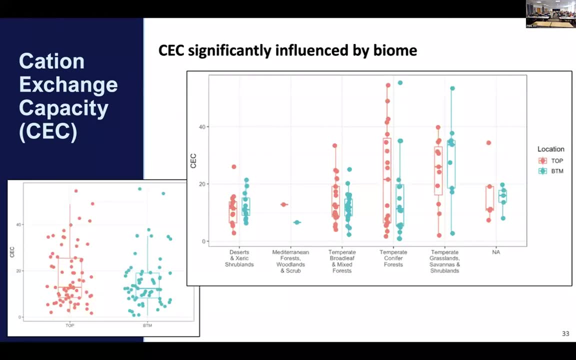 Maybe we'd see similar trends because we saw those were correlated. Or maybe we'd have a little more carbon in them. Not sure We need to look at some of the strengths tomorrow. What drove CEC? CEC was not influenced by depth. 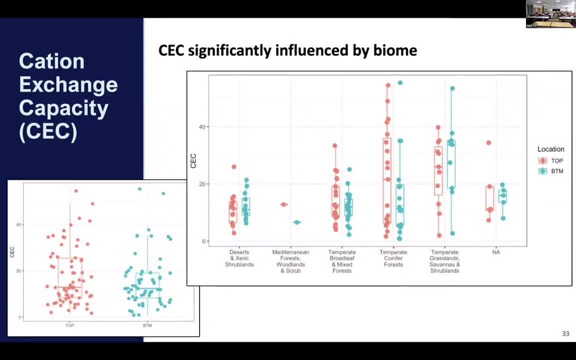 So top versus bottom, no significant difference in these samples, But there was a significant difference by biome. So again we see some trends: Desert versus temperate versus Mediterranean forest. We see some differences in these biotimes. So those are some of our gains. 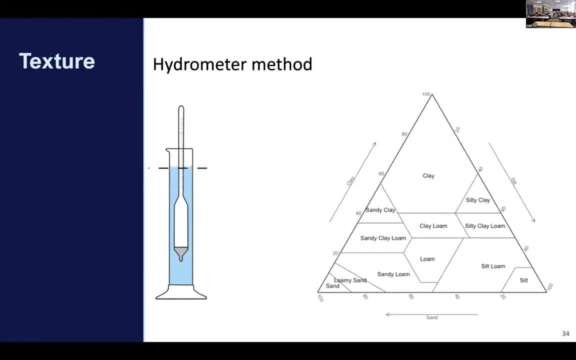 Our final technique that I'm going to show here is soil texture. This was using the hydrometer method- Again, basic soil physics method. Many of you have probably used this. The hydrometer measured specific gravity measurements at different points And that will give us the percentage clay. 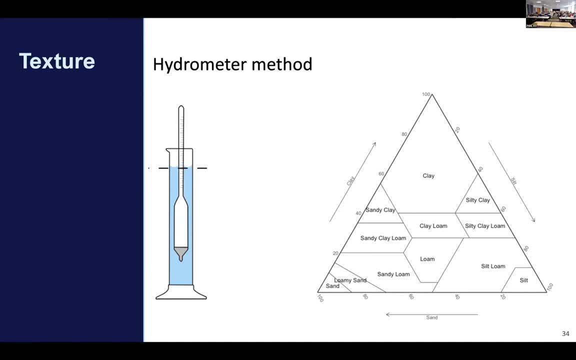 We then take our soil sieve, that through a 53-micron sieve to get the percent sand, We have percent sand, percent clay. The difference from 100 will give us percent silt. We throw that onto a soil texture triangle or this ternary plot. 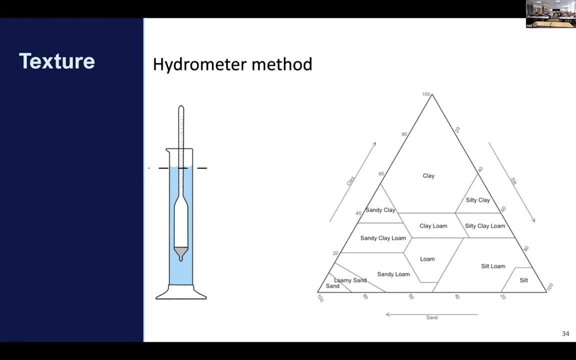 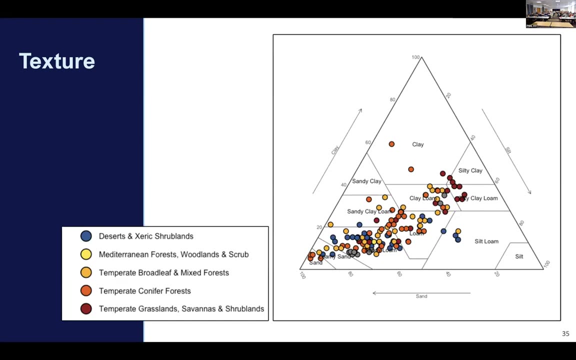 and we can use that to tell us what our soil texture is. So that was just the blank, just a blank triangle, and here I populated this with our samples that are colored by the biome types And if you squint, if you look closely, you might see some trends separating out. 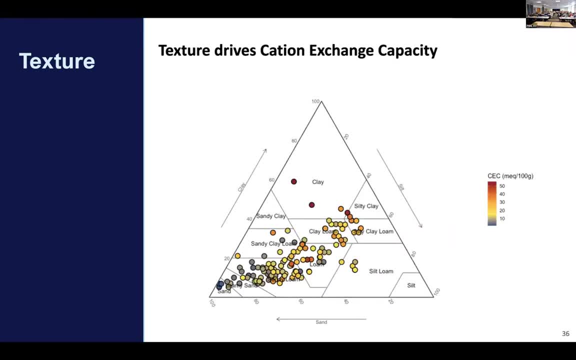 But, as we've seen, percent, clay and CEC were highly correlated. So here I've taken the same data points and colored them by CEC And you can see. if you go from sand up to clay you're actually seeing a trend of low CEC towards high CEC. It's not very clean. 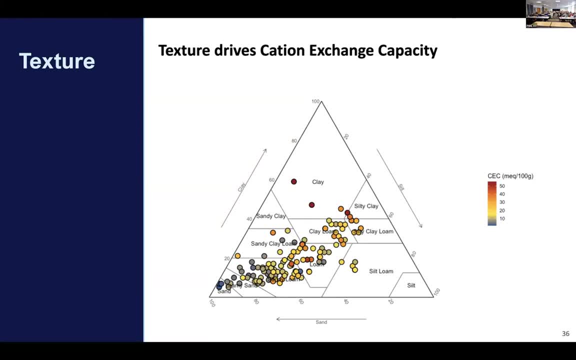 but you can see there's a lot of blue here, going into yellow and orange and all the way up to red. So this is another way of visualizing some of these trends. There's definitely something going on here And, of course, if you're interested in specific sites, we can take a look at those tomorrow. 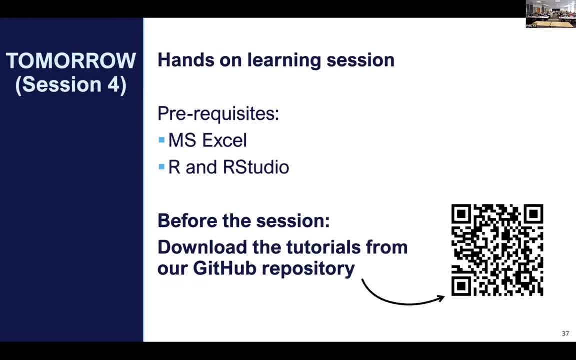 All right, So that's all I have for today. Hopefully this excites you to look into the data some more. Just a plug for our session tomorrow We'll be doing these one hour hands-on sessions. Chen and I will be handling that, Chen will be doing the respiration And. 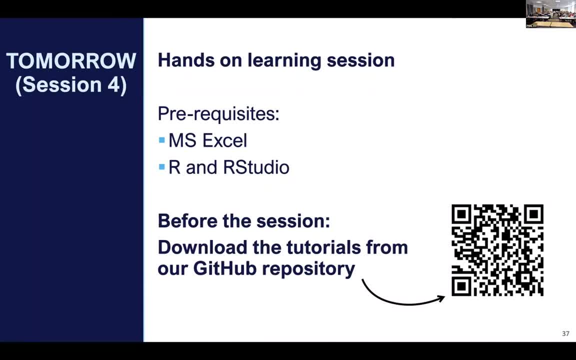 for that we ask you to come and load it with Microsoft Excel. We need a specific add-on. We'll be doing a solver add-on And on the GitHub we've provided instructions on how to install that. For my portion, I recommend R and RStudio, just because that's what I've been using, But of 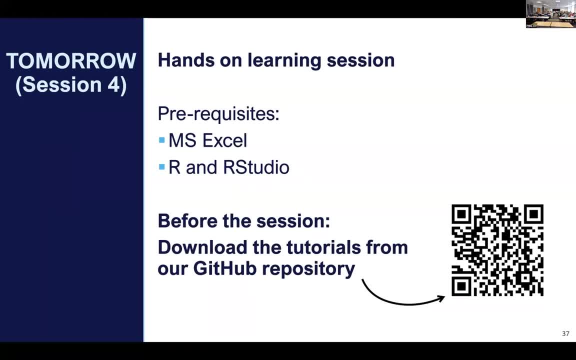 course, the data are available in a CSV format. So if you're more comfortable with Excel, that's fine. If you're more comfortable with Python, that's also okay. It's basically whatever you find useful. We'll use those to make some graphs, look at some data And, of course, we've got some tutorials available. 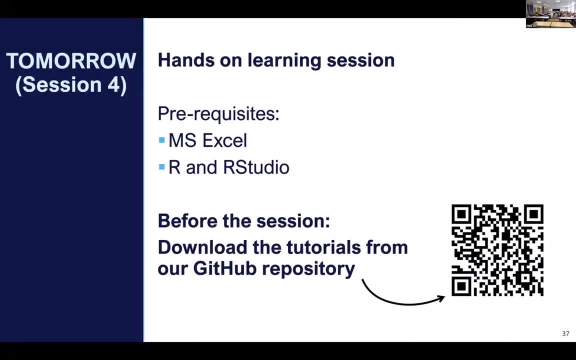 And of course, we've got some tutorials available. And of course we've got some tutorials available On the GitHub repository. you can follow the link through this QR code. It'll take you to those tutorials. Download those ahead of time. They have instructions on. you know what needs to be done. 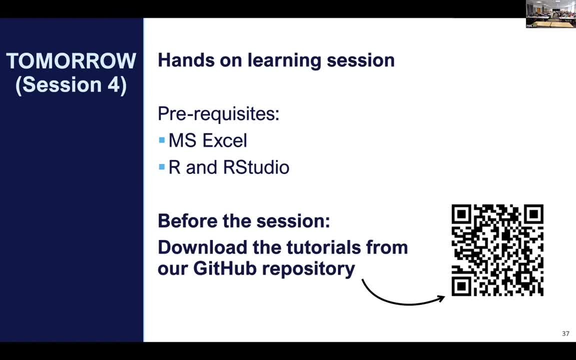 If you're using R, you might need some packages. Just get those downloaded and then we'll start that right and early tomorrow. All right, that's it from me. I think it might be a little early. I don't know. if anybody has questions, We can try and answer right now. 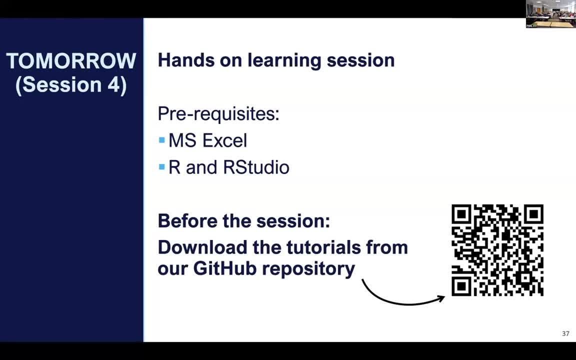 So I have a question about total carbon. Do you measure the organic carbon inside or just the total? Just the total, Because in those dry environments you have a lot of the organic carbon inside That may not represent Right. What do you want to see? I think for this one we did just the total carbon. 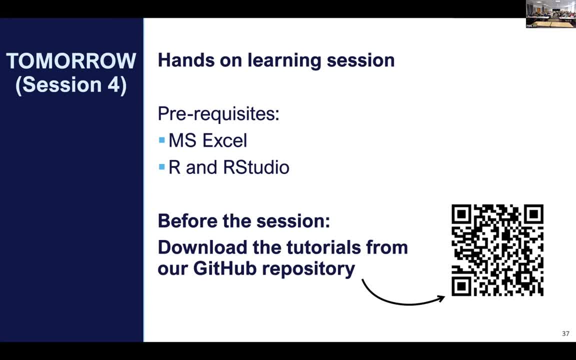 And then organic was only on the, on the soluble fraction. I don't know if for future iterations, if we're going to look at organic versus inorganic, Inorganics could be more than 50 percent total carbon in dry environments. Very important to differentiate. That's something we are. we have been looking. 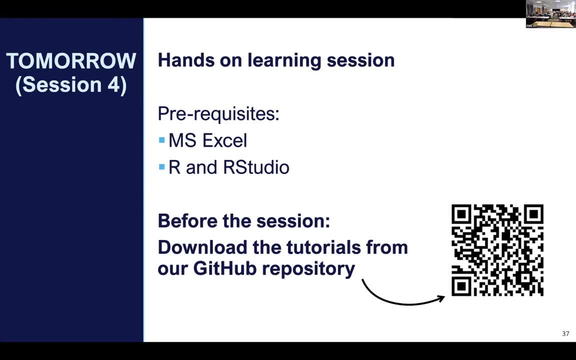 into those protocols. It is a lot more involved because it involves acidification of your samples and then processing them. So that's why we didn't do it for the pilot, But that's something we're thinking of, maybe for future, future campaigns. Yeah, but they can be measured simultaneously. 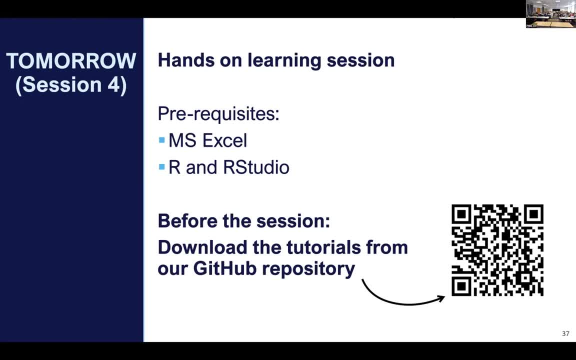 on the same time with a TOC. But so, yeah, I think we should and we will take it into consideration. Okay, Is there an analytical record on the samples Standard error or deviation? Yes, I believe it was done in triplicate. 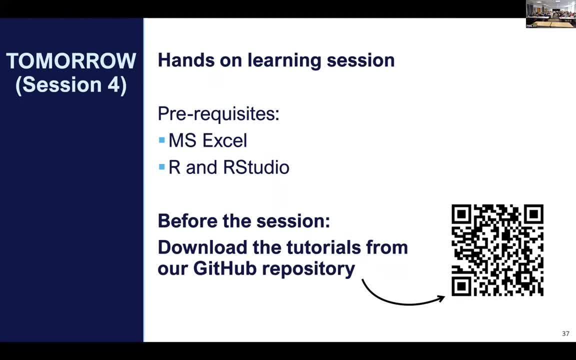 And here we've. I've shown only the like, the summaries, the mean values, but the actual data set online on Zenodo has the standard errors and standard deviations. Do you do any like organic matter treatment for your texture? I did not handle that part of the lab. 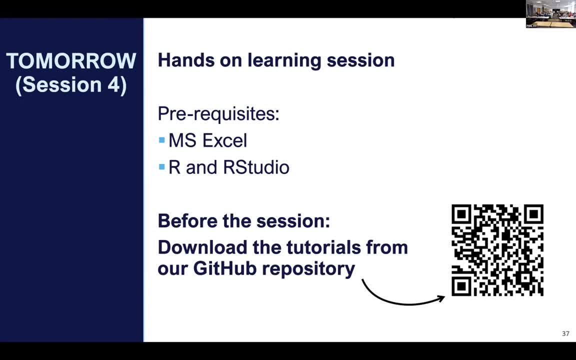 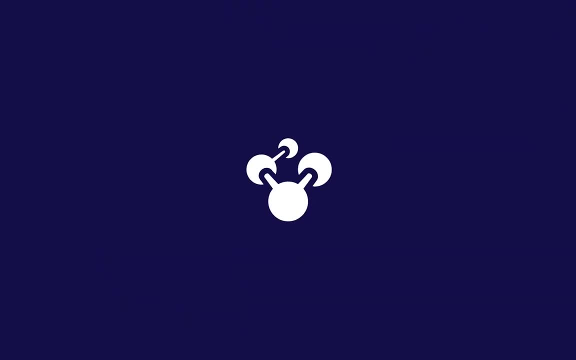 Okay, My third treatment on texture. Yeah, but we're doing that, I don't. I don't think we did Like. this was one of those things where it's you know where you've got a hundred samples. you have to. you have to make compromises somewhere, So we decided not to do that. 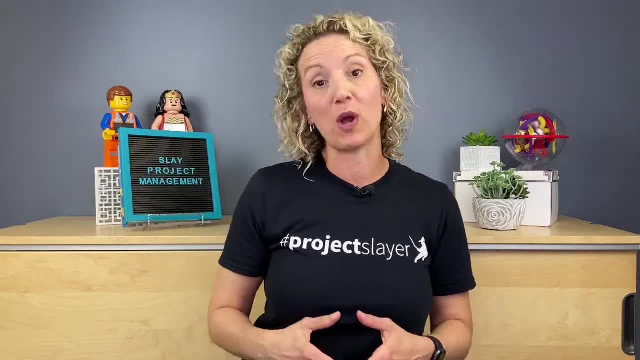 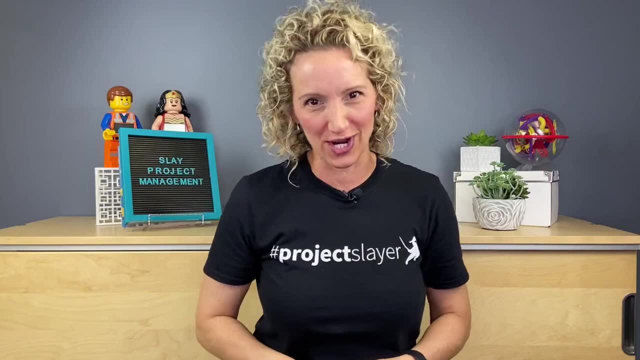 Are you getting ready to bring a project to close and you're wondering about closing out the project? Well, in this video, I'm going to share with you the tried and true techniques you need to close out your project. And if you want to become a project ninja, stay tuned to the end. 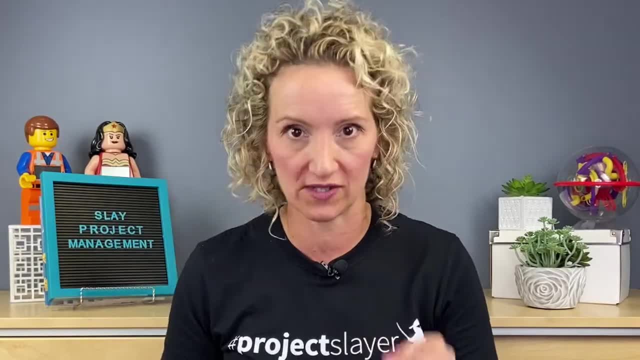 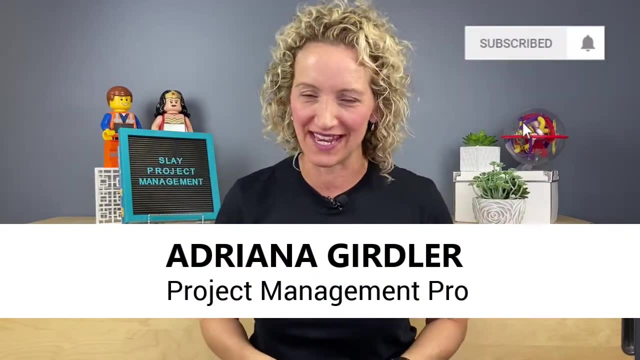 of this video where I'm going to share with you my checklist on why projects fail, something that you definitely need to know. Hi, if you're new here, welcome to the best career and project management advice that's going to come to you every Wednesday. I've managed countless of. 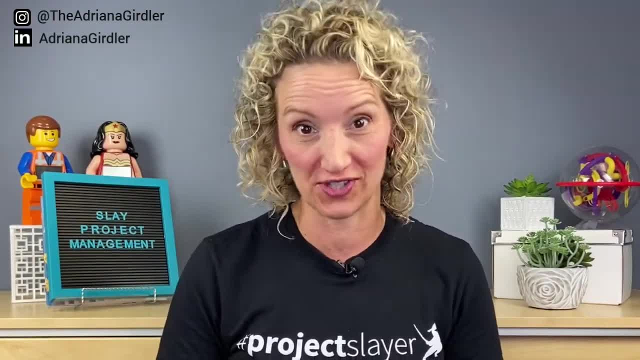 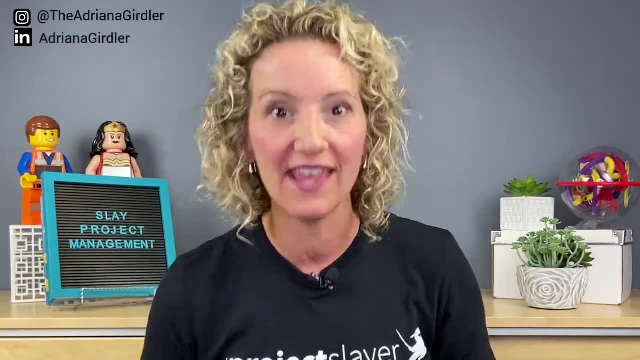 projects and closing out your project is critical to your success, And in this video, I'm going to share with you the top five tips you need in order to successfully close out your projects. Now, if you're excited about this, like this video, Double check The first thing you want to do. 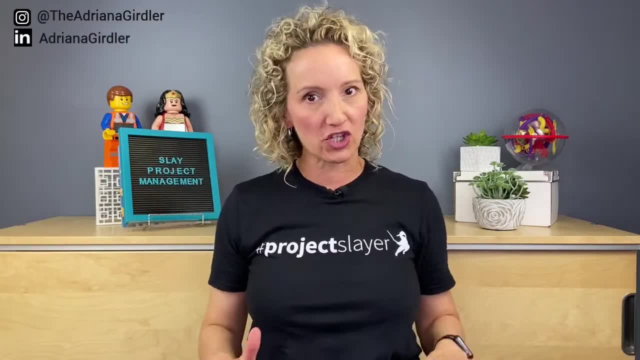 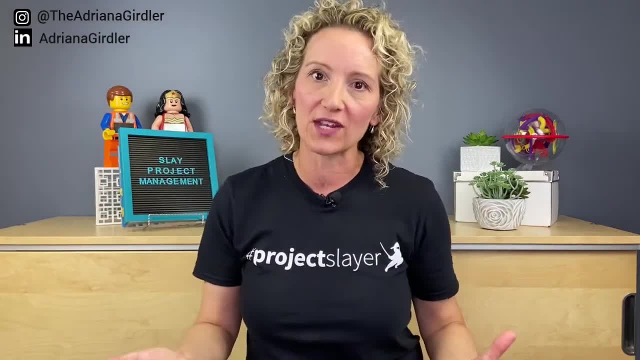 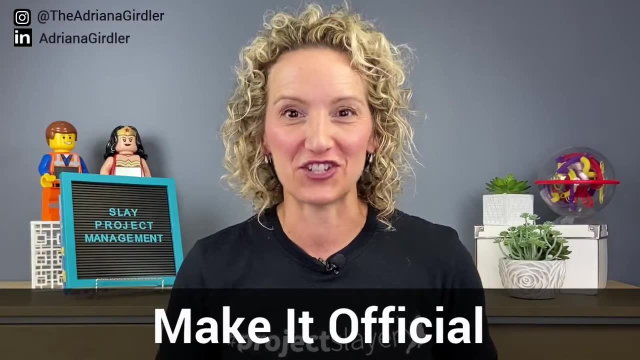 are focusing on the scope statement and that you achieve that deliverable. You want to check in with the sponsor, the steering committee, as well as the customer who is getting that deliverable. Make it official. It is really important that you declare, not just to your team, but everyone. 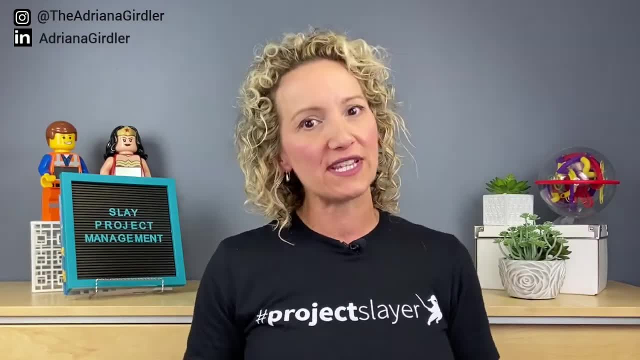 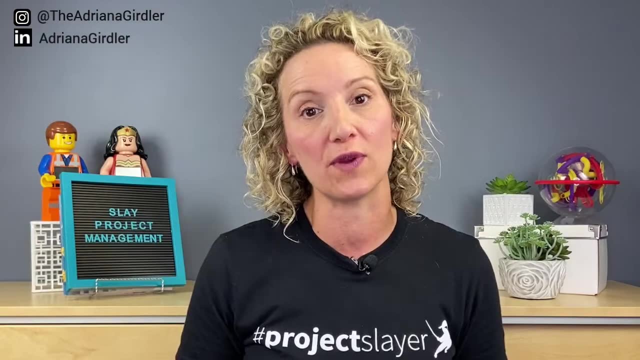 involved that the project is officially over. There's a couple of ways you can do this. One is to do an email blast to all key important stakeholders and anyone that you've communicated with regarding this project, both within the project team and outside of the project team. 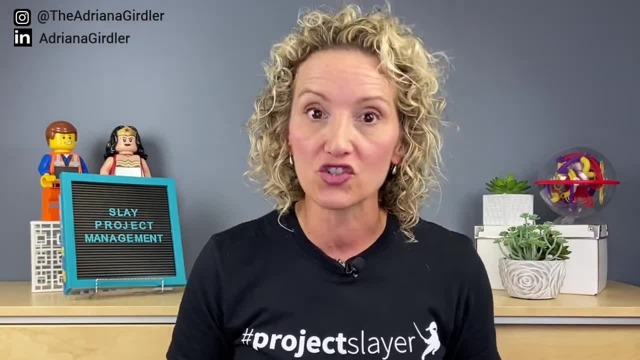 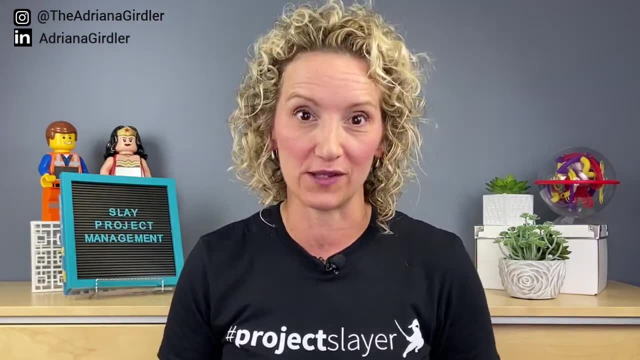 You also want to ensure that you close out any contracts, anything that is going to say this project is a close. And really important is you want to have a project celebration. This is a lovely way to really close out a project. It's quite interesting with large scale projects.